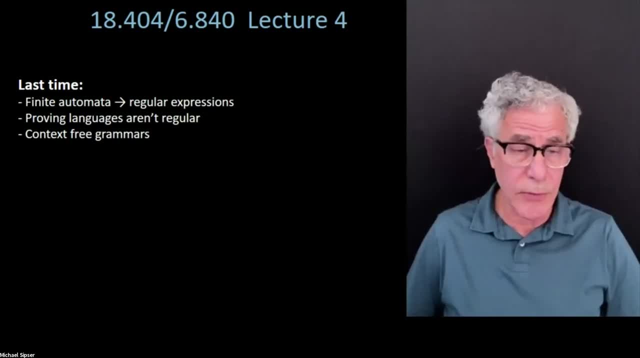 you can do. I think we saw that last time as well. There's some things you can do with context-free grammars that you cannot do with finite automata, And but they still have their limitations, as we'll see. So, today, what we're going to do, we're going to continue that discussion. 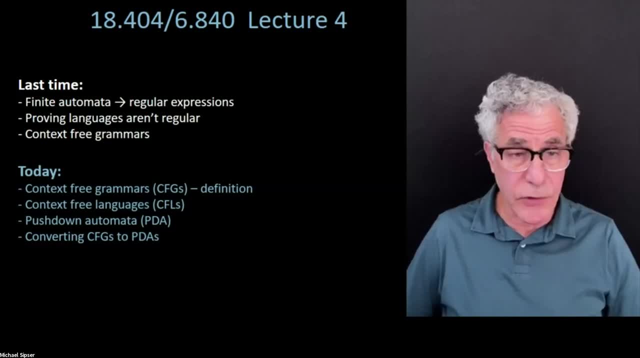 by looking at the definition of context-free grammars in a more formal way. One of the things that we do in this course is develop practice with formalism, And so that that's going to be in the spirit of that, We also are going to look at their associated. 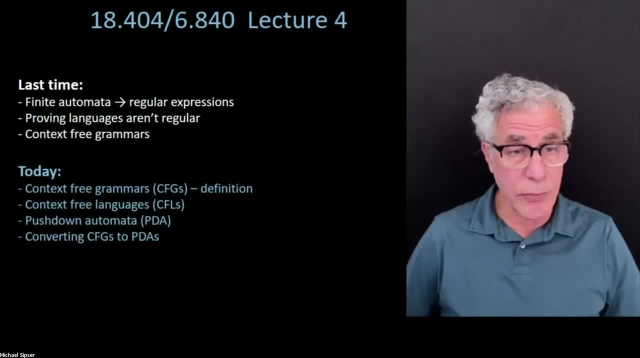 languages called the context-free languages. So they're going to be the counterpart for context-free grammars of what the regular languages are, for the finite automata regular expressions, And then we're going to look at an automaton-based model which is the counterpart. 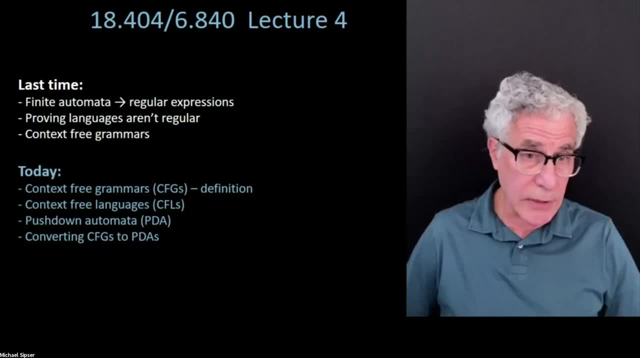 to the grammars called the pushdown automata, And we'll see that those are equivalent in power. And finally, well, and it's part of that, we will show how to convert the context-free grammars to the pushdown automata. And that's what. that's what. that's what we're going to do. 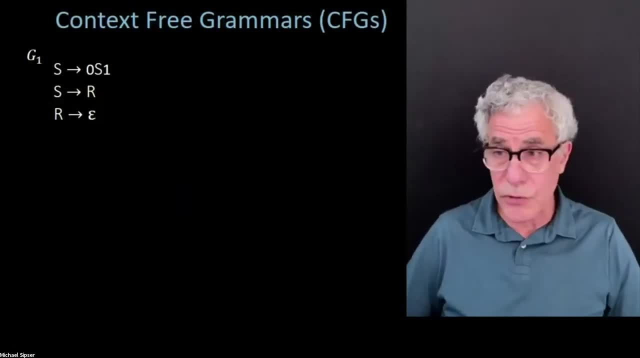 today. So we're going to move on then and return to our topic of context-free grammars that we began last time, And just to refresh your memory, So here was that example of a context-free grammar that we gave last time, And it has the way we're going to be writing context. 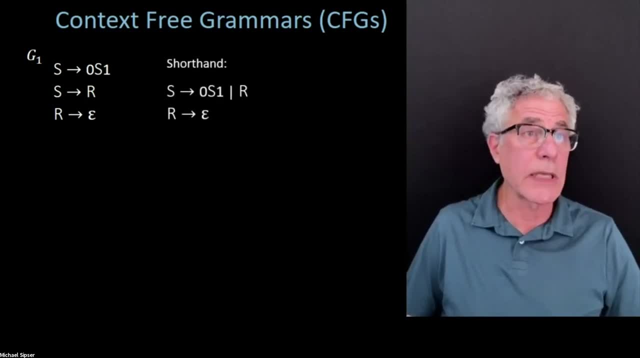 context-free grammars is using a bit of a shorthand, which looks like this: When you have multiple rules that have the same variable on this on the left-hand side, you can combine them into one line. So these two rules over here- S goes to 0, S1, and S goes to R- can be written. 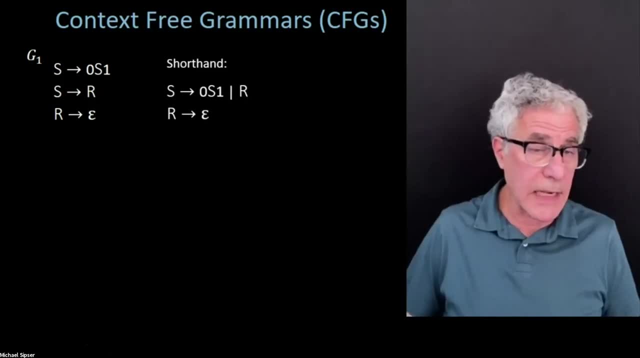 in one line as a little bit more compact way. This is standard, as S goes to 0, S1, or R. That's where you would read this. Only two rules, but written on one line. Okay. So, as you recall from last time, a context-free. 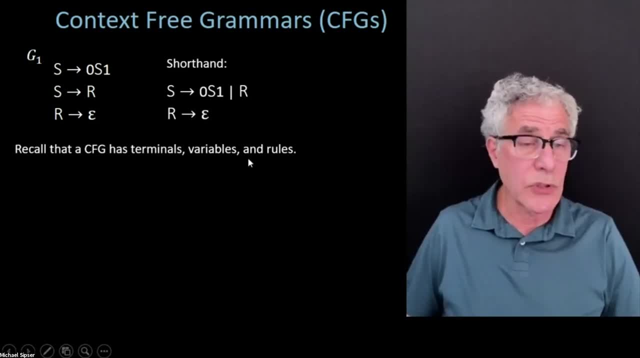 grammar has terminals, variables and rules. Those are the parts that we speak of, as well as one of the variables being designated as a starting variable, which gets the whole thing going. So I'll talk remind you about how the computation goes. But so the variables are the symbols that 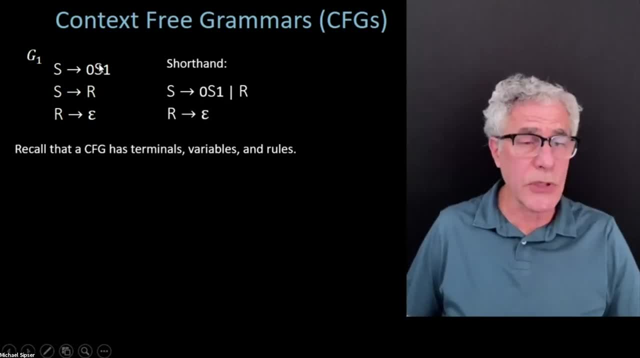 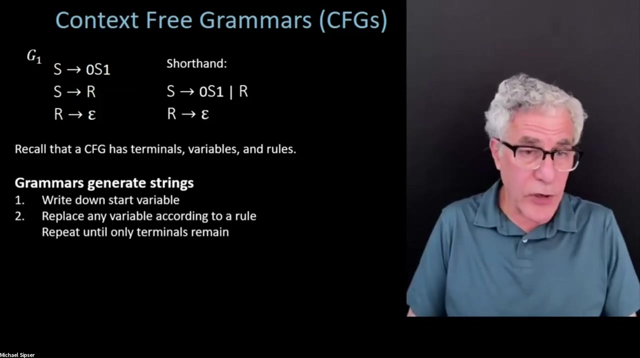 appear on the left-hand side of the rules. The terminals are the other symbols that appear in the grammar, And we take the grammar and we use it to generate strings according to a certain system, And the system is that you start out by writing down the starting variable And then, once you've written down that variable or whatever, 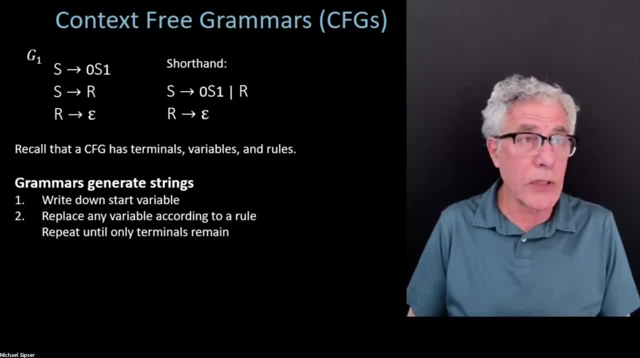 variables you have, you write down the starting variable And then, once you've written down that written down, you're allowed to substitute them according to the rules- the substitution rules- that are in the grammar. So you can keep on replacing the variables that you have with. 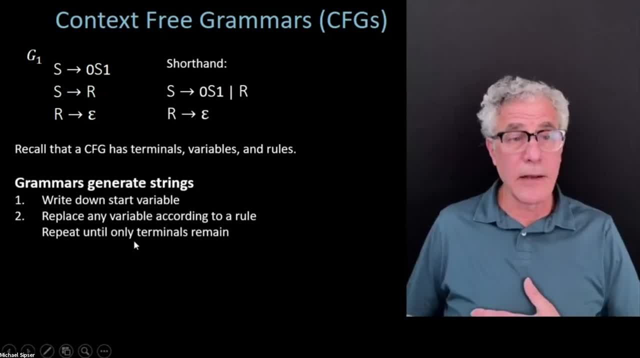 the corresponding right-hand sides, and then you do that over and over again until you don't have any variables left. only terminal symbols remain, And at that point you have generated a string that's in the language of the grammar. So the grammar's language is going to be: 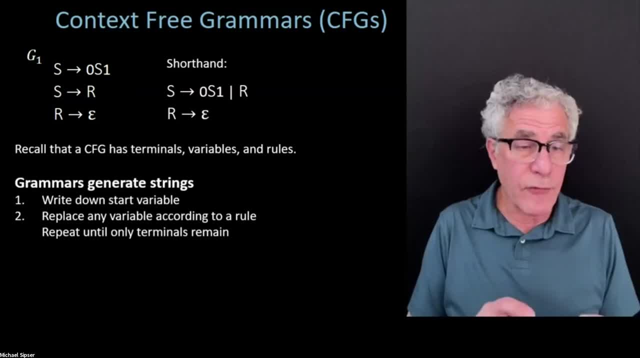 a language over strings whose alphabet are the terminal symbols. So the terminal symbols in a certain sense play the same role as the input alphabet, say for the finite automata. The variables are kind of internal working symbols For the grammar. the terminals are sort of the symbols over which the language is written. 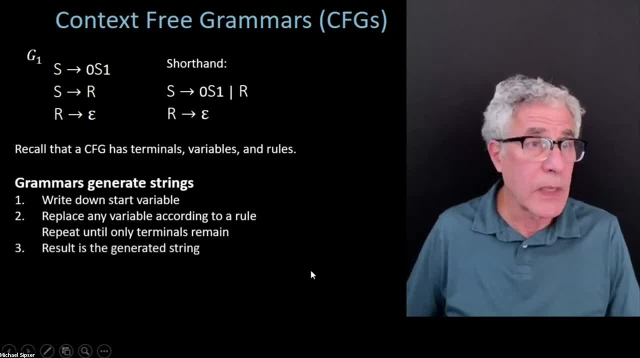 We'll make that more precise in a minute when I give the formal definition. So the result is the generated string and the language of the grammar is the language of all generated strings that you can get using that grammar. And the important thing is that we call. 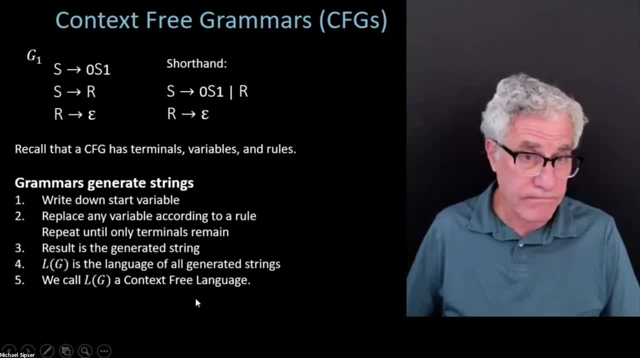 that language a context-free language, So that's like what we get from that. That's the analogous thing to the regular languages, but here we call them context-free languages- the things that you can get from a context-free grammar. Again, just a quick recap. 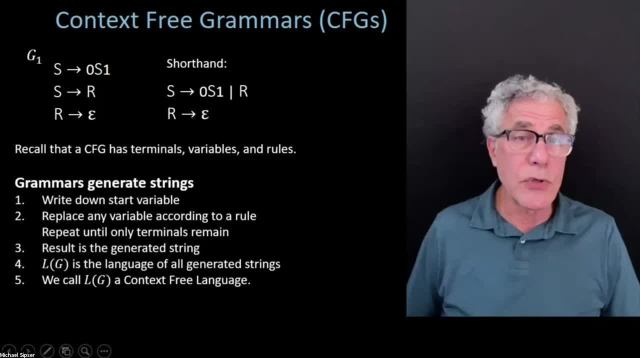 of that example we did last time. So you start out by writing the start variable and then I'm going to give you kind of two views of that, either in terms of the tree of substitutions, which we call the parse tree, or in terms of the resulting string, as you do the substitutions. 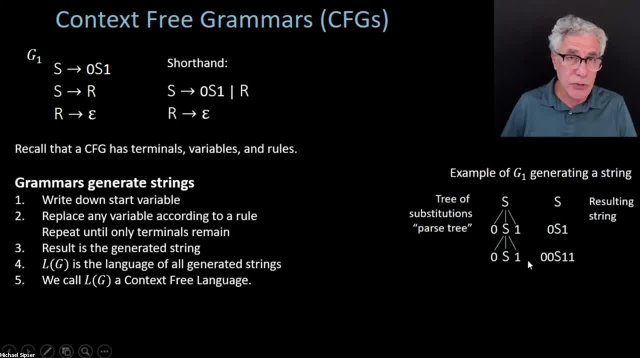 So here is the parse tree, Here is the resulting strings, Here are the substitutions that you make. And now we have R coming from S and we have 00R11.. And now we have R. in turn becomes an empty string, And then the string that we generated is 0011. 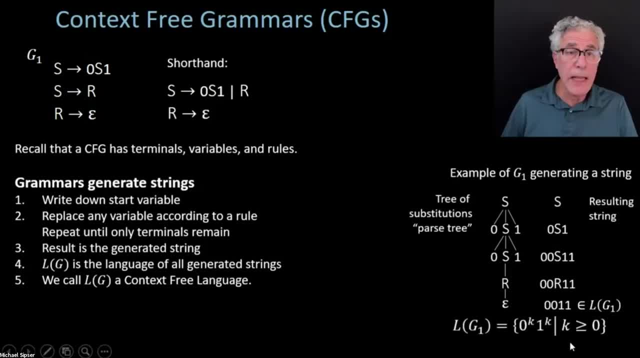 That's in the language of the grammar, And now, if you play with this a little bit, you'll see that the language of the grammar is all strings that look like runs of zeros followed by runs of ones. All right, So is that clear? 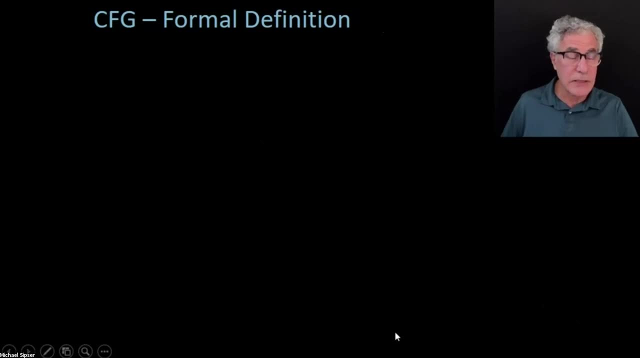 I think we're going to have a, I think the next slide is going to have a check-in, And so hopefully that'll get us all together on the same page with this, Anyway. so here's our formal definition. anyway, We have a context-free grammar. 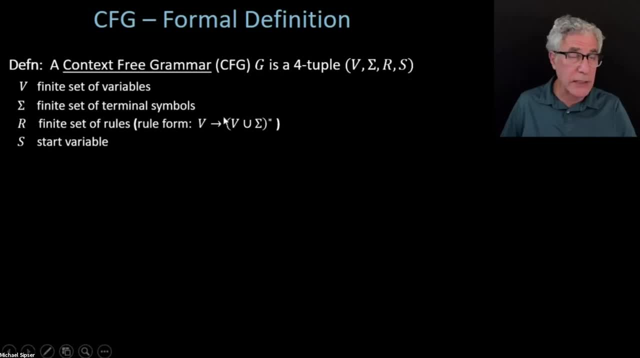 is a four-tuple. There are four parts to a context-free grammar. These are the parts we've already been discussing: The variables, the terminal symbols, the rules. the rules are always of the form a variable, followed by, you know, with an arrow, to a string of variables and terminals. 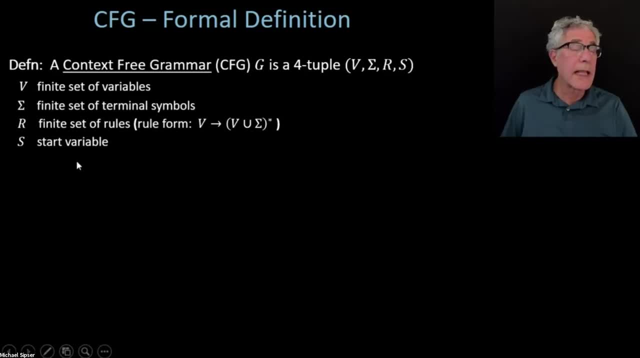 That's why we just write that down. So this is the form of the rule, And then we have the special start variable And we all wrap that up into a package. this four-tuple. That's what the context-free grammar is. 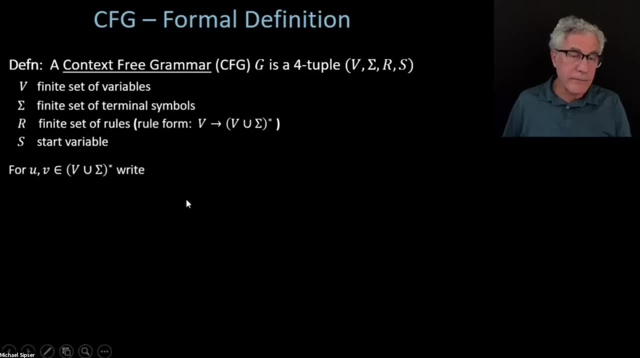 Now we have here and now maybe a little bit overkill, but let's talk about what, formally speaking, what the way the grammar actually processes and produces strings. So we're going to write: the standard notation for this is that if you have two strings of variables, 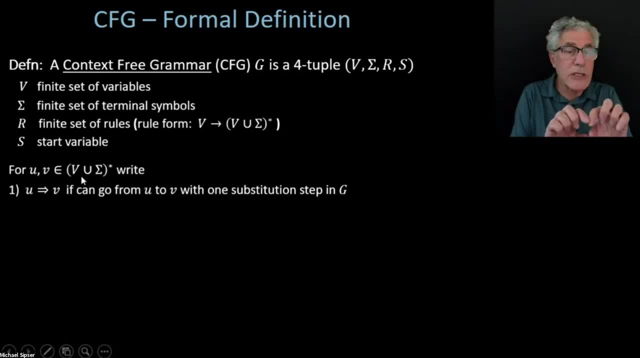 and terminals. So imagine you have an intermediate string that you've generated in the grammar so far Which might be like 00S11 from the previous slide. So that's an intermediate string. that is so far what you've generated. You're going to say maybe that's U and V might be the next line down. 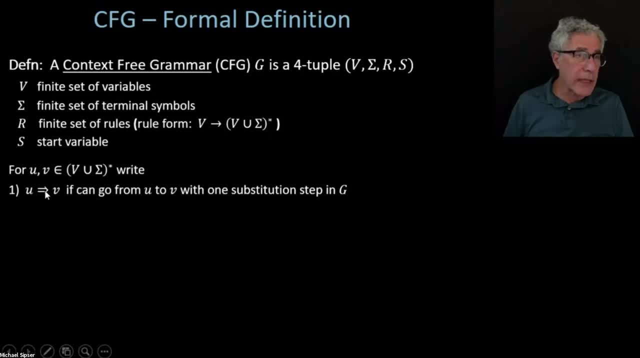 So that means we're going to write U, arrow V, and that arrow is The word we're going to use, is yields. We'll say u yields v if it can go from u to v just with one substitution step, And then we'll write u yields v in some number of steps, or actually we say u derives v. 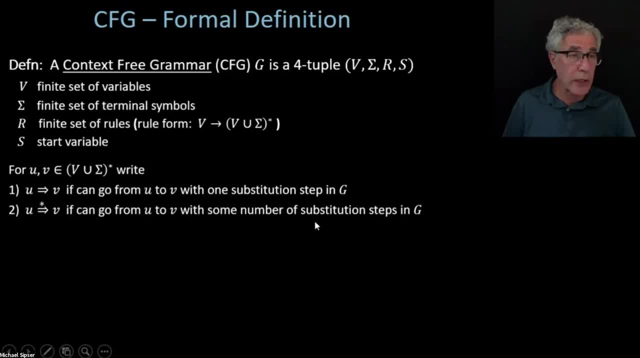 if it can go to u to v with some number of substitutions instead of just one, And that's used with the yields arrow with the star above it to mean some number of Another way of writing. that is, you can say u goes to v if there are a bunch of one-step moves. 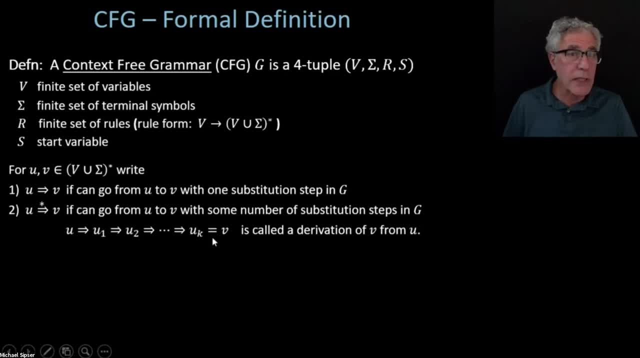 that you can make which take you from u to v, And that whole sequence is called a derivation of v from u. That's a sequence of steps that you go through, doing these substitutions one by one, to take you from u to v, according to the rules of the grammar. 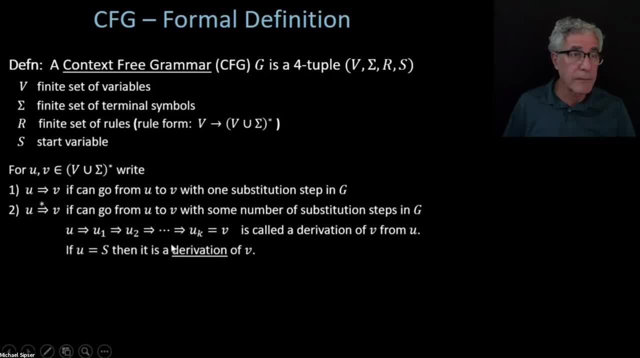 And lastly, if u is a starting starting variable, then we call that sequence just the derivation of v. It could be the derivation from the start variable, but that's kind of the assumed if you don't say it's a derivation from anything. the derivation of v. 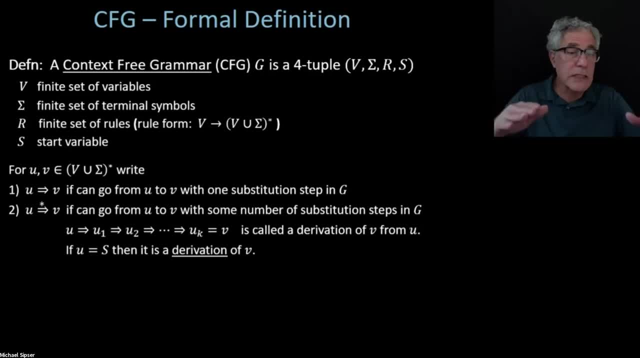 in the grammar is the derivation of v from the start variable. It's just the sequence of substitutions that you make, Kind of the you know what you, what I think you would expect. Now, the language of the grammar is the set of all strings that. 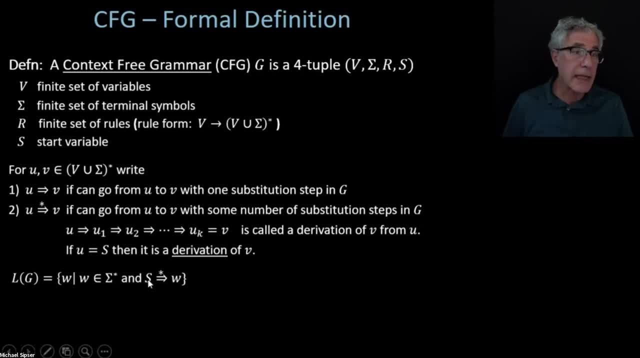 of terminal symbols that you can get from starting at the starting variable of the grammar. Okay, and that's called a context-free language, as I mentioned before. So it's a context-free language, It's the language of the grammar. for some grammar. 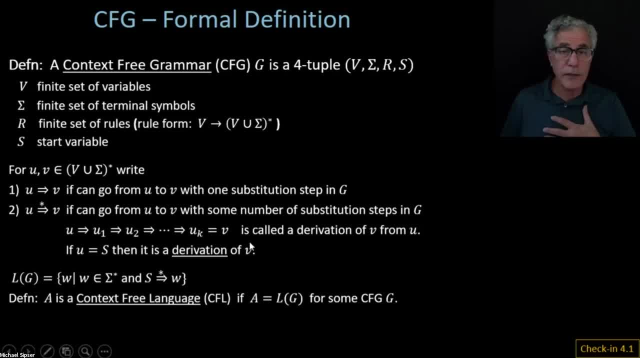 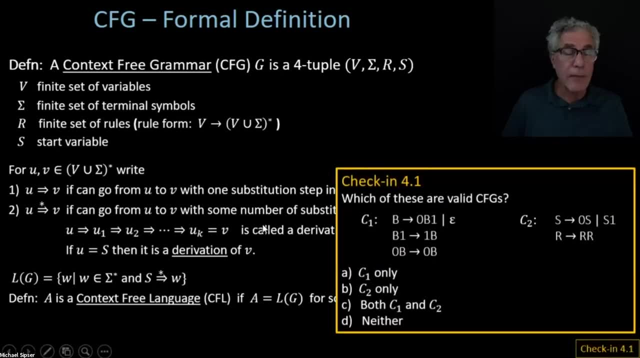 Okay, so let's have a little check in here Again. nothing too hard, nothing to get worried about. anyway, We're not counting correctness here, So let's just see. I'm going to give you two things that look like grammars. 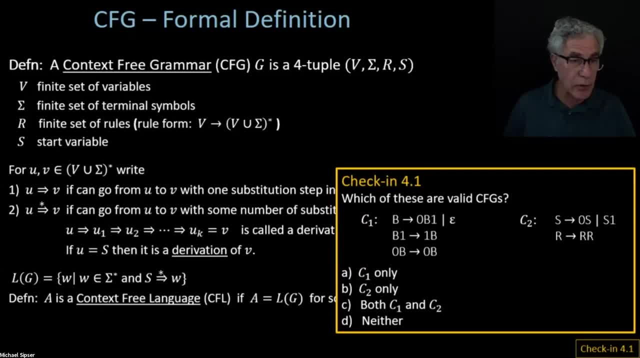 Which of them are actually grammars, And let me just pull that poll up here. Okay, so which of these are valid grammars here? Are they both? Neither? I mean you can kind of make an argument either, you know. either way for both of them. 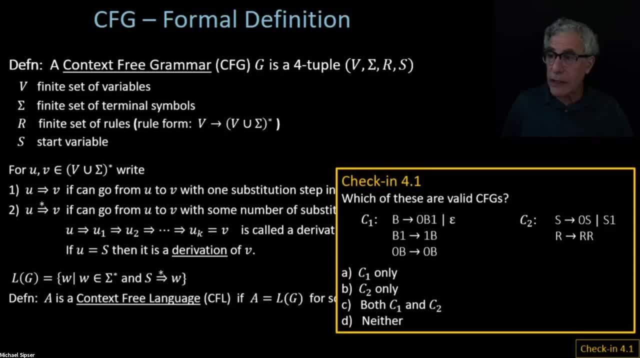 But both of them are kind of a little, have their own, a bit of weirdness to them in a way. If you, if you, if you study them for a second, Okay, that's pretty much converged. Share the results. 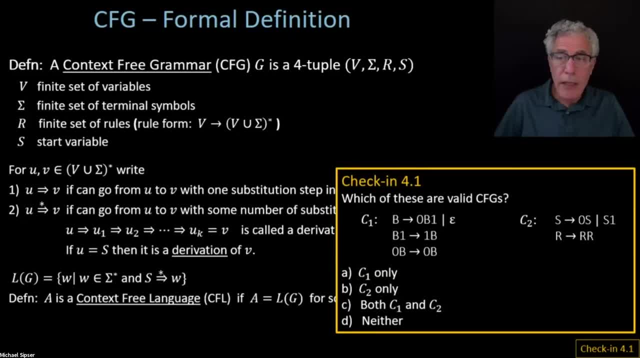 Okay, so. so in fact, the correct answer is B. And why is only C2?? Well, first of all, you know well what's wrong with C1? C1, the problem with C1 is that the rules have things besides a single variable on the left-hand side. 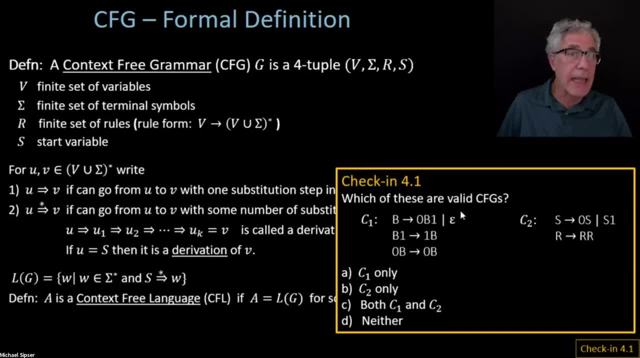 So having a B1 on the left-hand side is not legal in a context-free grammar. In fact, there are other kinds of grammars. There's a kind of grammar called a context-sensitive grammar. The term context-free means you can replace the variable independent of its context in the intermediate string. 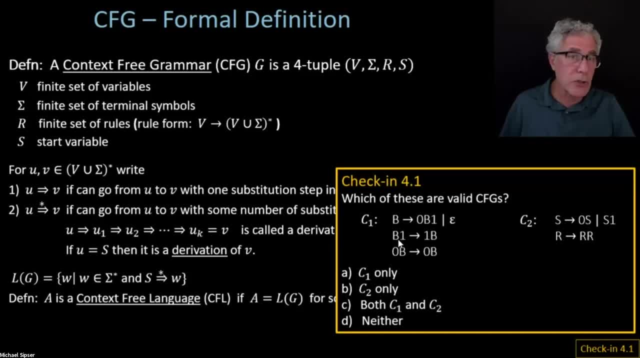 So independent of what's around it. But here this substitution is going to. you can replace B, but it depends on there being a one next to it. This is called a context-sensitive grammar, but it's not the kind of grammar we're going to be using, which are only context-free grammar. 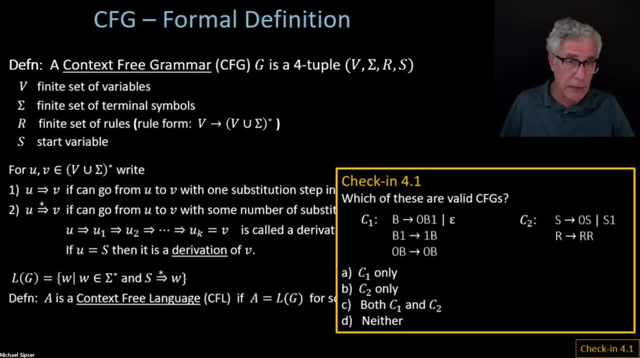 So C1 is out. That's not a legit context-free grammar C2,. the thing that's a little weird about C2 is if you try to generate a string in C2, you'll see that there's no way to get rid of the variables, that you're always going to be stuck with a variable. 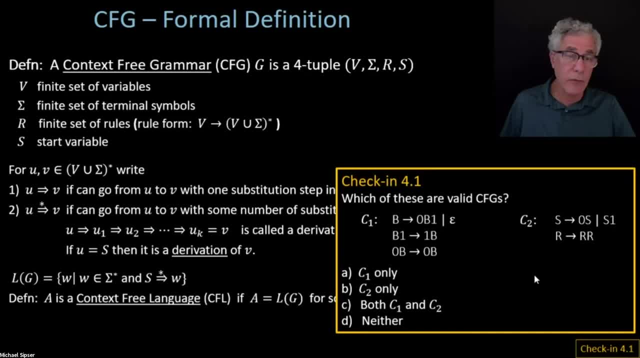 Now that doesn't violate the definition of a context-free grammar. So this is a context-free grammar, but it's not going to be able to generate any strings of, only terminals. So this is a context-free grammar whose language happens to be the empty language, but that's totally okay. 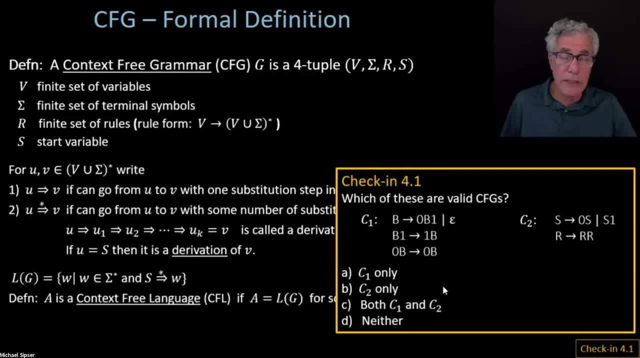 So the correct answer here is B, That only C2. here is a valid context-free grammar. Okay, Common, let's just see. common question: does a string u derive itself? Yes, a string u derives itself. That's a little bit of a little bit of an esoteric question there for us right now, but yes. 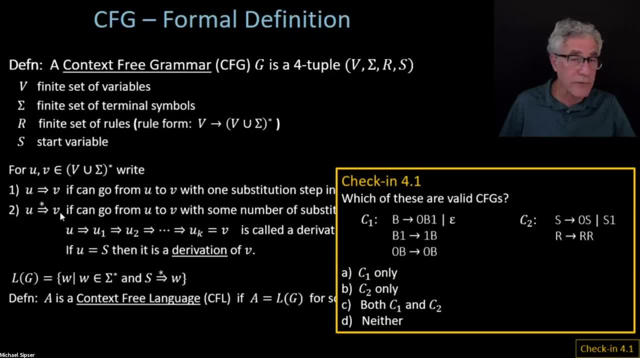 A string, u in this definition here u arrow stars, u is legit- is legal. Maybe it isn't According to the way I've written it down here, but it is. it is a legal thing. It's not going to really matter for you anyway, but but it is legal. 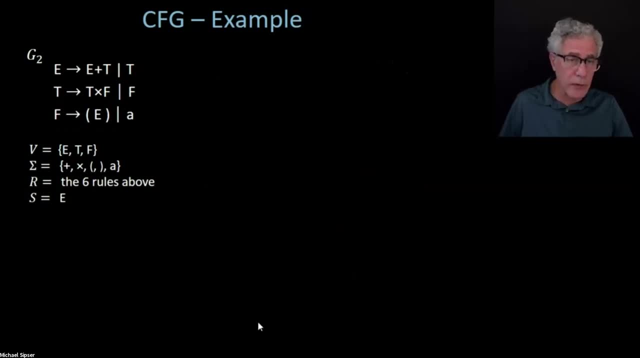 Okay, let's continue. Let's do another somewhat interesting example of a context-free grammar. This is a grammar that is, can generate arithmetical expressions involving pluses and times. So here it is. It has how many rules? Well, there are six rules. 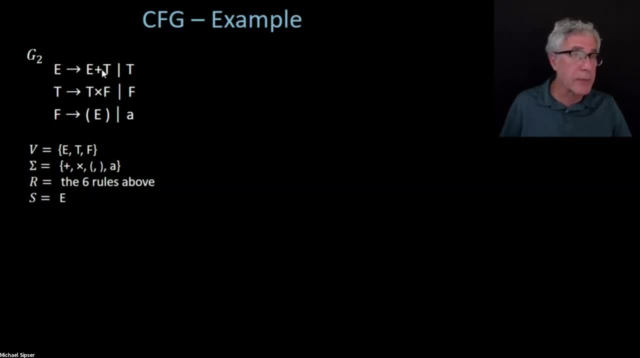 There are six rules here. Each line represents two rules. So e goes to e plus t or t, t goes to t times f or f, and f goes to parenthesis, e, parenthesis or a Now. so the variables are going to be the symbols that appear on the left-hand side: e, t and f. 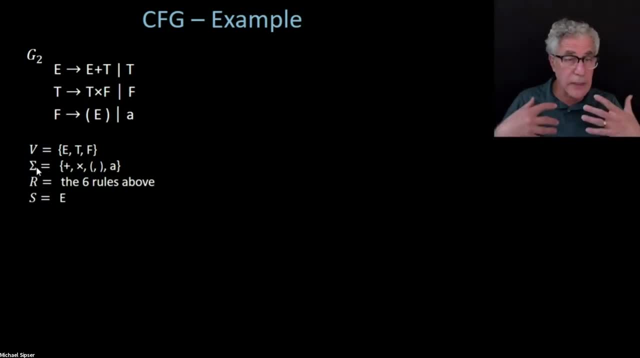 The terminal symbols, which are going to be the symbols of the language that you're going to be generating, is going to be the plus, the time symbols. The parentheses are just terminal symbols here, So they're nothing not playing any special role besides that. 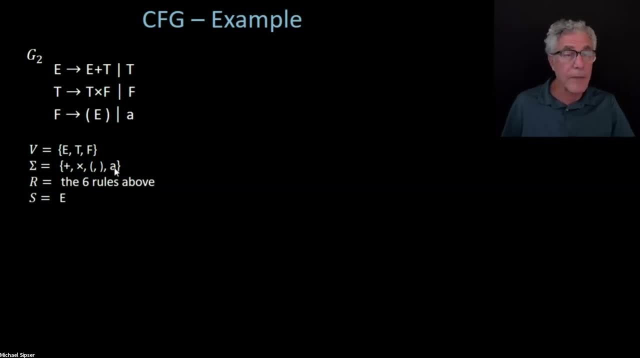 And then you have the a, which is representing kind of the operand on which those operators would be working if there was actually an expression you would use. But they're just symbols from the perspective of the of the grammar. And, lastly, the start variable is going to be as normally appears, on the upper left-hand side of the grammar, in terms of the way you write it down. 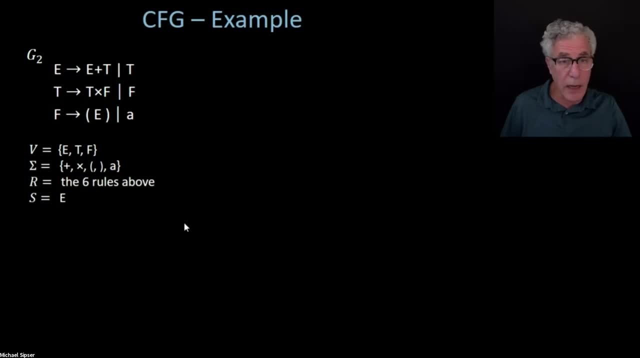 So sometimes you might specify a different start variable, but otherwise, if it's not specified, it's that it's the one in this corner here. Okay, so let's just see some examples of using the grammar to generate a string. So here is a string in the language a plus a times a, and this example will kind of reveal some other interesting features of the grammar. 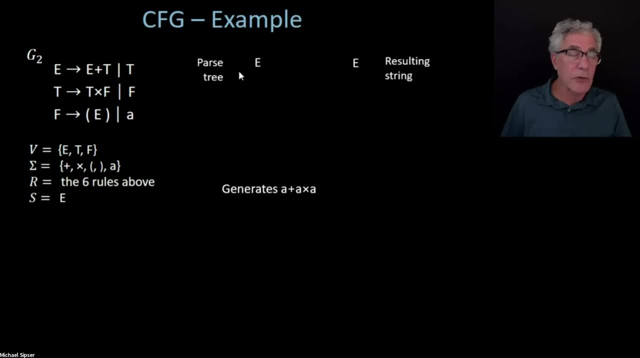 But let's just see it in operation first. So again, I'll try to write it to you in both ways, In terms of the parse tree and the resulting string, as you're doing the substitutions, So the. so first we start with the e that we substitute e plus t and we see the resulting string is e plus t. 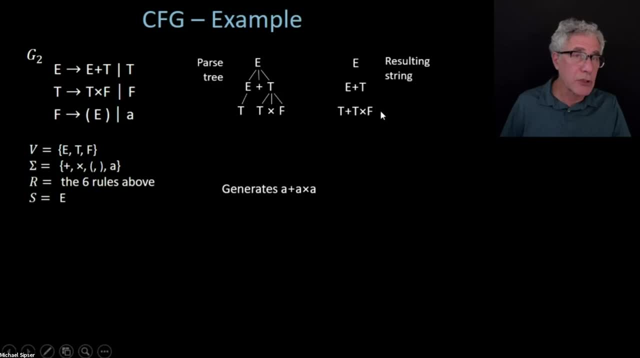 But now we, as we're doing additional substitutions, the resulting string that you get is going to evolve accordingly, And so I hope it comes across that this tree here picture on the left shows you the structure of the various substitutions, whereas on the right it just shows you the strings that you get as a result of those substitutions. 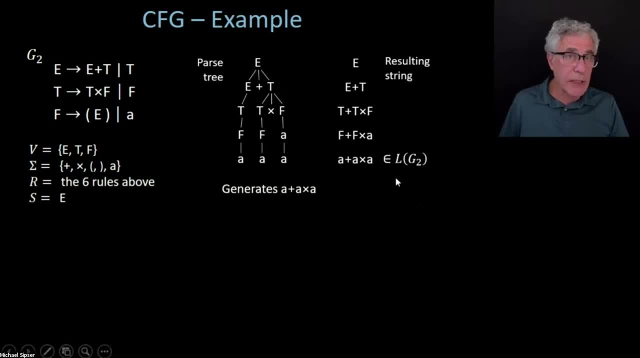 So now you can generate this particular string, which is now in the language of this grammar. You could generate all sorts of other strings as well, such, as you know, parenthesis a plus a, parenthesis times a, and so on, And in fact, this might be a piece of a. 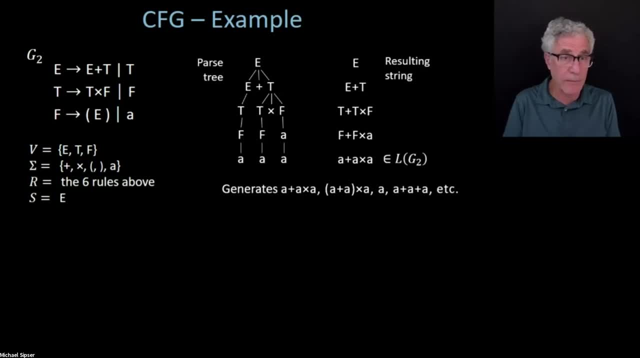 programming language that you're trying to describe, And one application of context-free grammars is to describe the syntax of programming languages. You know what are the legal programs that you can write with in that programming language, And not only that, the grammar can be used to automatically generate the part of the compiler. 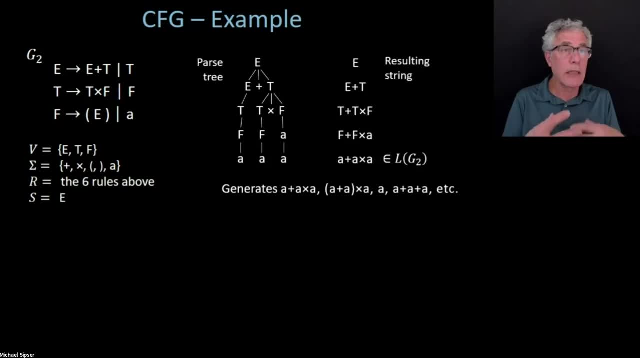 for that programming language Which will interpret the, which will interpret the structure of the input. you know, the so-called parser, which will figure out the meaning of the input to the compiler, so that the compiler then can generate the code or, if it's an interpreter, can interpret the resulting code that you've given it. 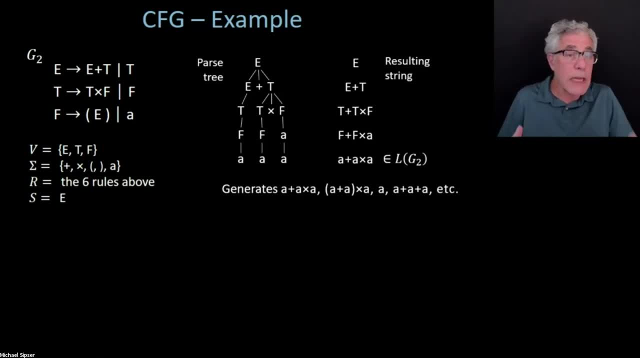 But the very first step in both of those is to figure out the meaning, And the meaning is is embedded within the structure of the parse tree. Now, in the case of this particular tree, just to give you some sense of what meaning I have in mind, 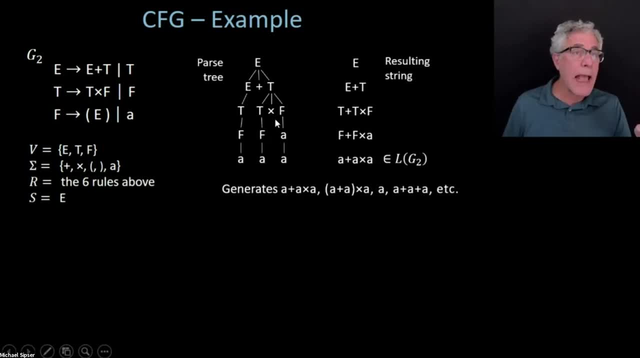 this parse tree, due to the structure of this grammar, has the precedence for times over plus. So normally when we write down a plus a times a, you assume you're going to do the multiplication before you do the addition, even though it appears. second. 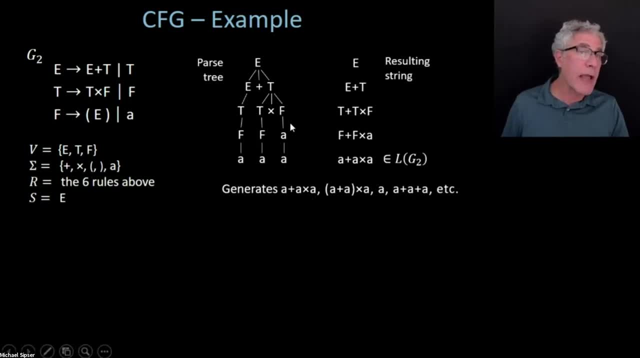 That's just the way we tend to write things And this grammar has grouped it that way for you. It groups the times lower down in the tree than the plus, So the times is going to be done before the plus, if you imagine doing this in terms of the way. 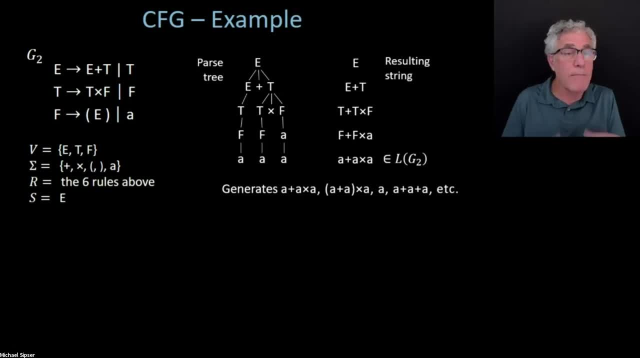 the tree is guiding you. So the tree, as you can see, has a certain amount of meaning built into it. Now, we're not actually going to be using that in this course, But I just want to describe that as an illustration of how. 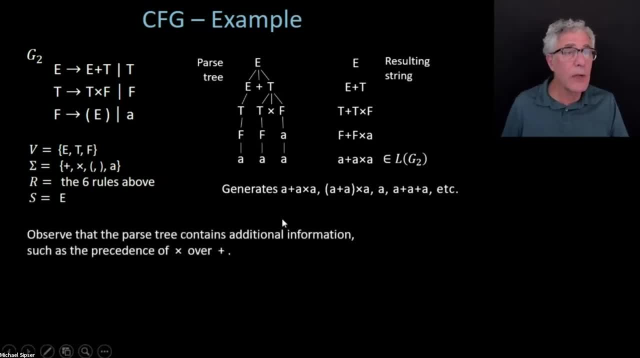 this material can get applied Now. so here is what I'm saying: that the tree contains additional information. Now, that's also relevant. if you happen to have a grammar which might allow multiple parse trees for the same string, That can happen. 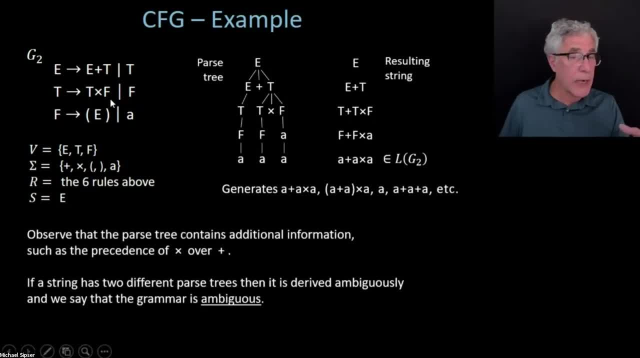 This particular grammar does not allow that, But you might write other grammars, as we'll see in a minute. that could generate the same string in multiple ways with multiple different parse trees. Now that might be undesirable when you have a programming language, because typically you want it. 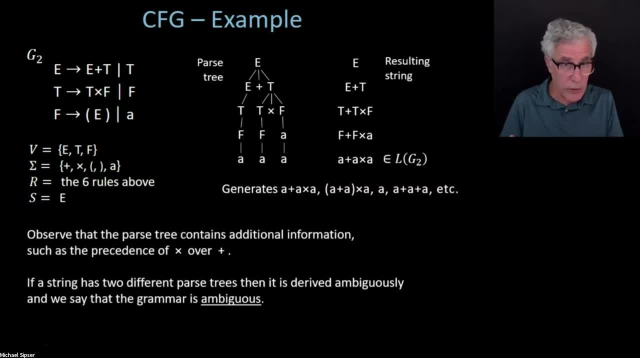 to be only a single meaning for your code. You don't want it to be ambiguous and have multiple meanings. But ambiguity does occur And it's not necessarily something we're always going to see as a bad thing. So I think, as I mentioned last time, 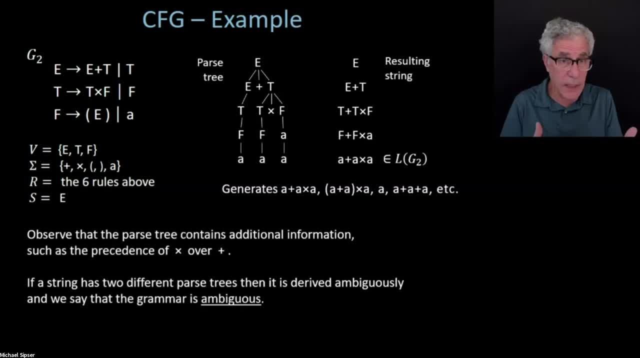 a lot of this subject originated with linguistics And that's where the terminology comes from: grammar and languages and so on. The terminology for the subject really comes out of linguistics. In fact, one of the key players for that is an emeritus faculty member at MIT, Noam Chomsky. 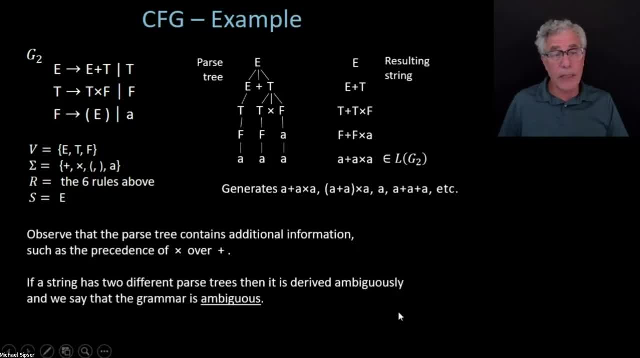 He was instrumental in setting a lot of this stuff up, But the you can think of grammars as applying to natural human languages as well, So let me give you a little example as a pop-up. It's not directly a pop-up- check-in. 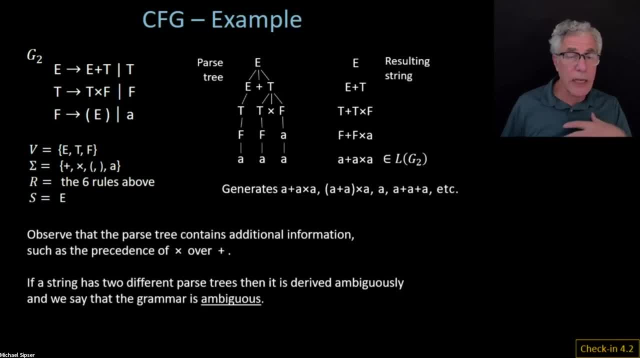 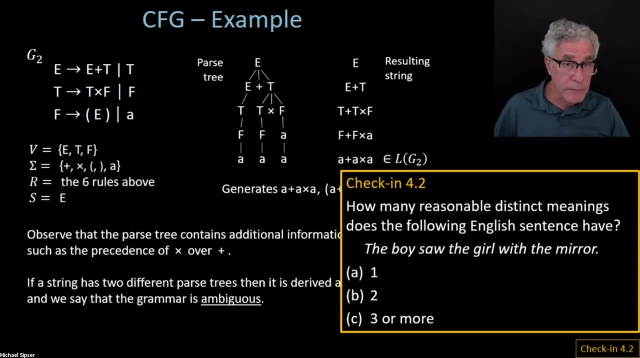 not directly relevant to the material I just presented, but just sort of a curiosity. If you take the English sentence, the boy saw the girl with the mirror, Is there only one natural interpretation for that sentence or are there perhaps other natural interpretations for that sentence? 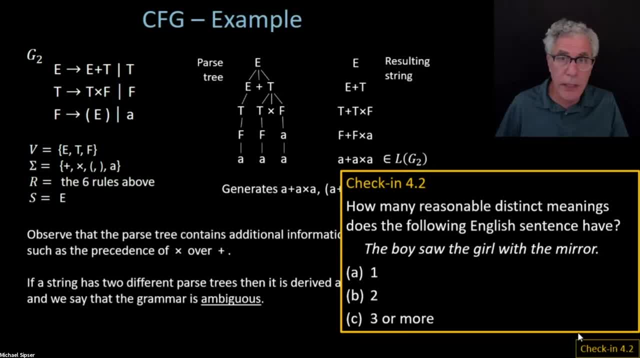 So let me pose that to you as another poll here. So I ask you to think about how many different meanings you might find for reasonable different meanings. I mean you can think of it as a whole if you're going to go wild. 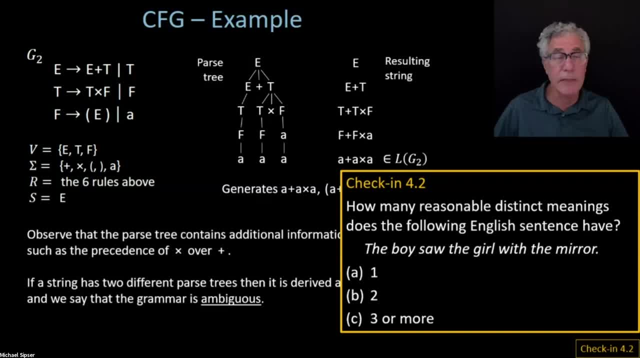 you can think of zillions of meanings, but I think in terms of reasonable meanings, how many meanings might you get for the sentence? People are seeing more meanings than I'm seeing, but that's okay. So this is quick. Why don't we just give this another 10 seconds here? 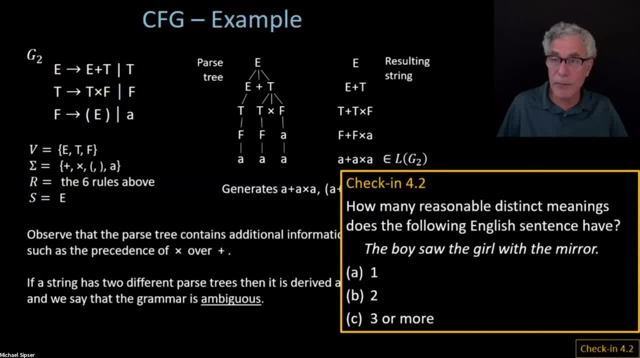 And then most of you are in agreement with me. I can see here that you are seeing that there were two meanings. The two meanings that I see here for this sentence are when you say: the boy saw the girl with the mirror is who has the mirror. 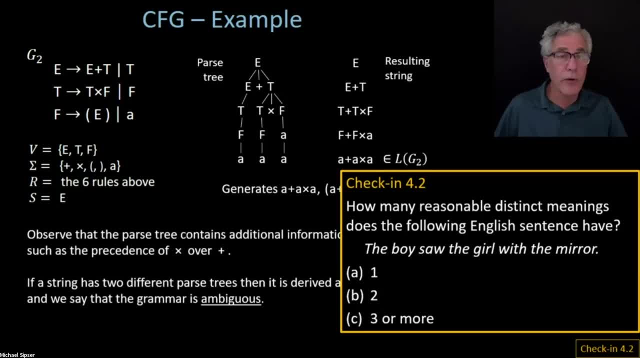 Is it the boy seeing the girl through the mirror, Or is it the girl that has the mirror and the boy just happens to see her? So two very different meanings for the same sentence, And that's what the the nature of English is. just the way. it's an. 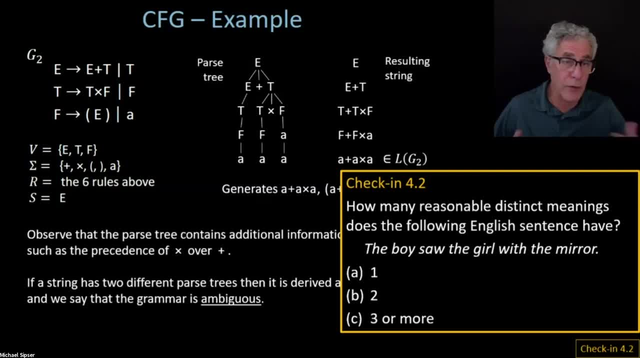 it's an ambiguous structure there And often we resolve that ambiguity in English with other information that we might have. But typically you don't want there to be ambiguity when you have this, a grammar, say, describing a programming, programming language, Okay, 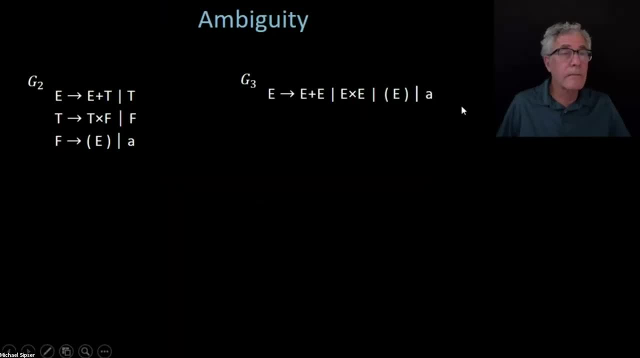 So let's continue on then. So, talking a little bit more about ambiguity, I was promised you an example where you might have an ambiguous grammar. So if you take these two grammars, G2 and G3, G2 from the last slide and G3 is a similar grammar- 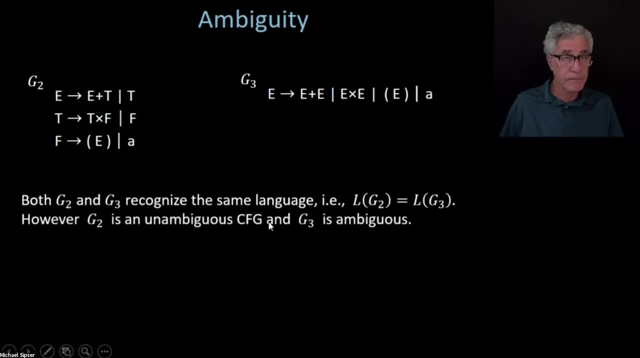 In fact, it's the grammar that has the very same language, that gives you the very same language. So L of G2 equals L of G3.. Both of them are describing these arithmetical expressions, But whereas G2 has a unique parse tree for every string that you generate, 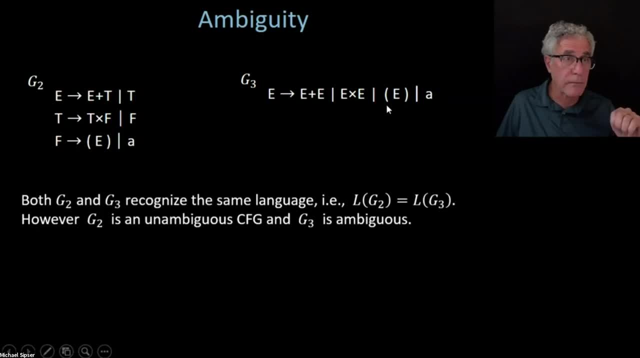 G3 can have multiple parse trees for the same string. Okay, So I'm just going to illustrate that here. So here is the same string that we generated last time- A plus A times A In G3, the parse tree is actually even simpler here. 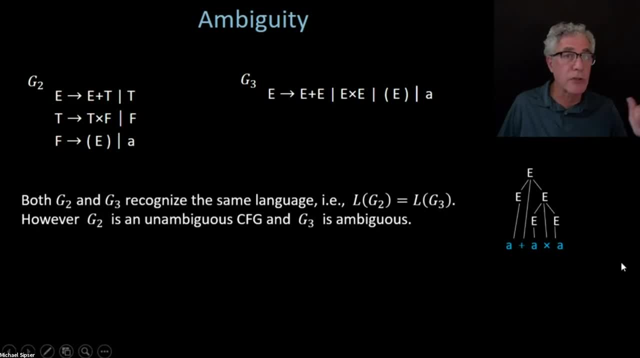 So here I'm showing you the just the two substitutions that you need to make, starting from E and then to get the string A plus A times A. It's a simpler grammar in a sense, But there's another parse tree that'll give you the same result. 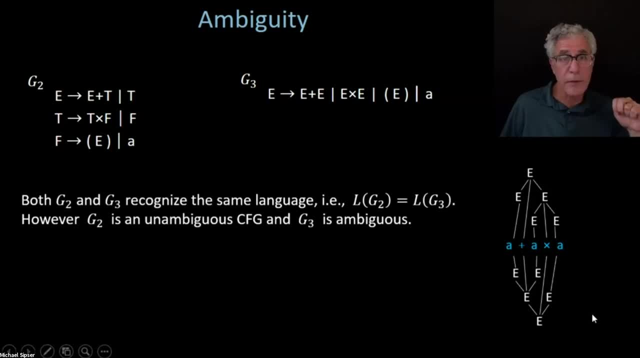 And I've written that down below here, upside down. So the upper parse tree groups the times before the plus more inside than the plus, but the lower parse tree doesn't have that precedence built into it and can alternatively interpret the plus as being of higher precedence than times. 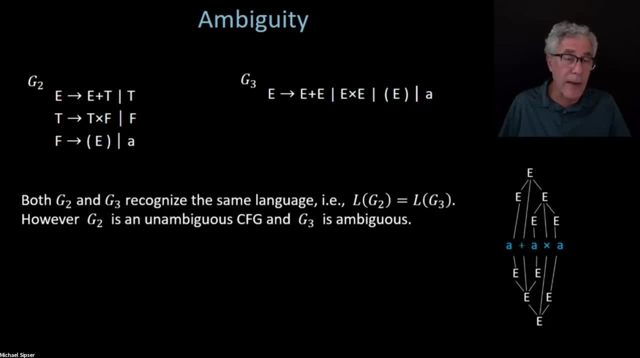 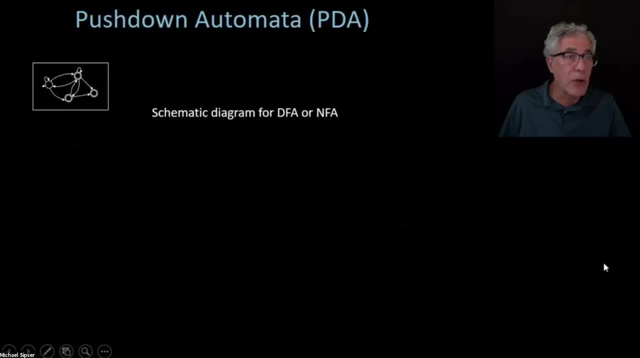 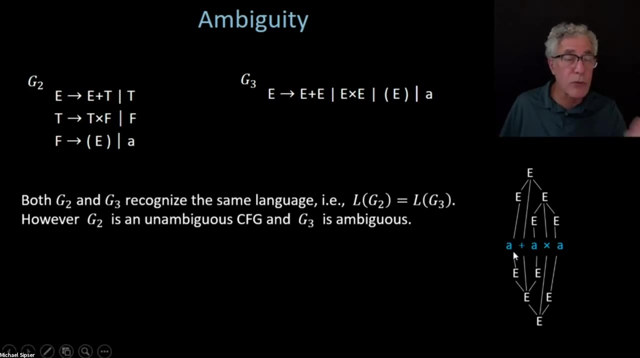 And so in that sense we have here a grammar which has two interpretations for this same string, and we call that whoops, we call that an ambiguous derivation, ambiguously derived string, and the grammar itself is called an ambiguous grammar. Okay, 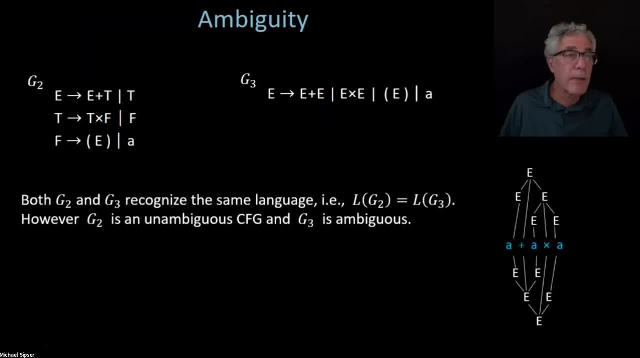 So let us continue on from that. By the way I there's a question here that came in like, for example, A plus A. is that ambiguous in G2?? No, If you, if you try to apply it, you'll see the way that G2 can produce A plus A. 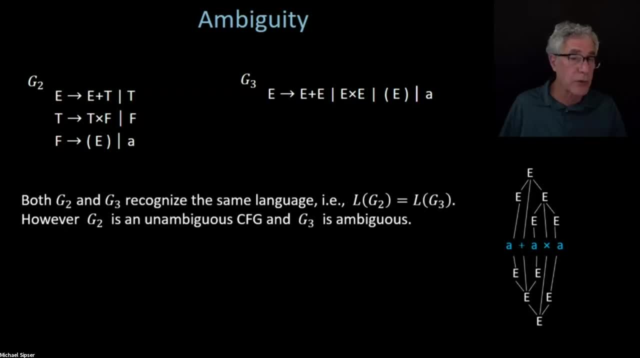 A plus A plus A is going to group the first two And then the, and then the second one, then the, then the last one. you can't, you can't derive things in multiple ways. I mean addition is associative. 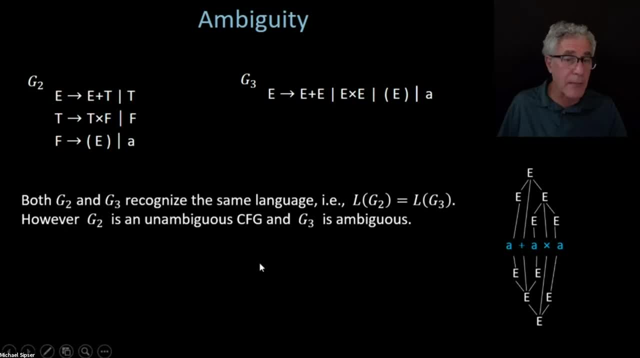 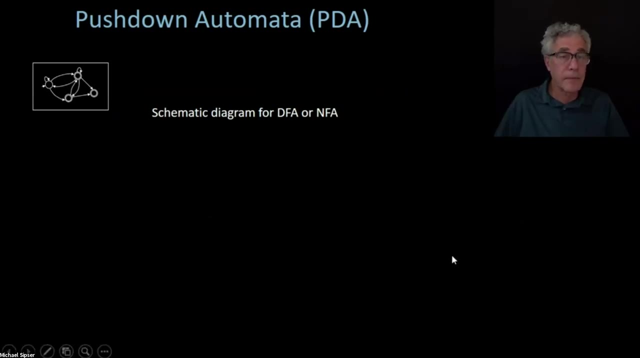 but the grammar doesn't. it doesn't the grammar for the grammar? it's going to have a prescribed order for the way things get interpreted there. Okay, So that's the ambiguity. So let's introduce pushdown automata, which is going to be our automata counterpart for context-free languages. 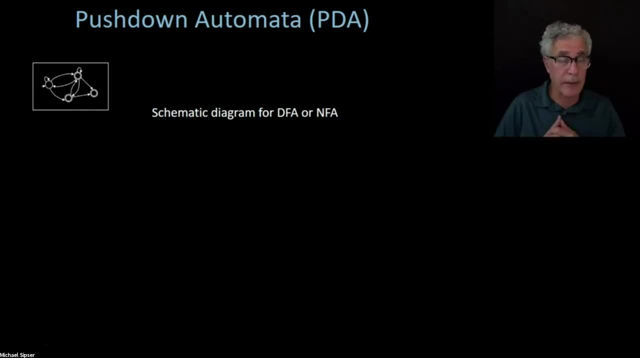 All right. So the way I'm going to introduce pushdown automata, sort of shifting gears here and now, is by first giving a new view of finite automata. Remember, before, when we presented a finite automaton, we gave it in terms of a state diagram. 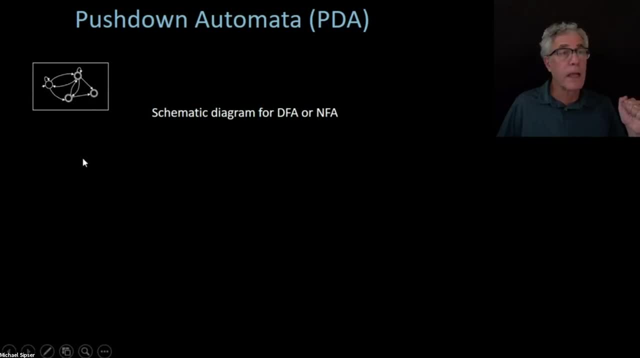 which I've kind of shown here in miniature form on the picture. We could do that for pushdown automata, but the picture tends to be very complicated, So I'm going to take a bit of a higher level description for pushdown automata. 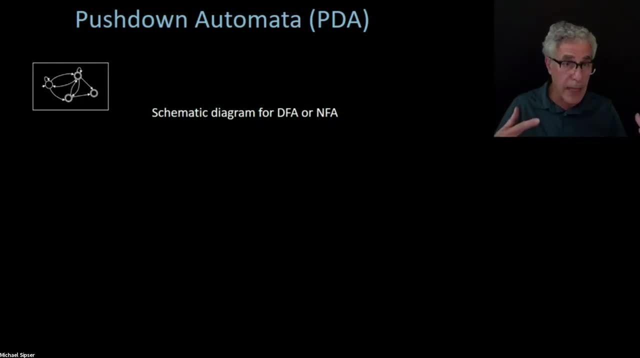 which is I'm calling a schematic view or a schematic diagram, And there I'm really not going to be showing you the individual states, but I'm going to be showing you the individual components of the machine at a sort of more of an abstraction and from a more abstract perspective. 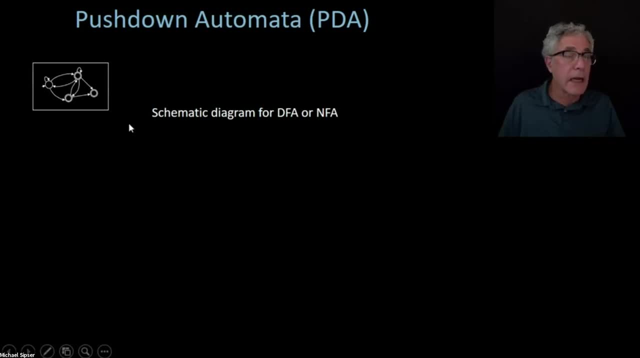 And so, from that perspective, a finite automaton has here what I'm going to call the finite control. So I'm going to be suppressing the details of the states in this picture. I'm going to represent that those states as the control of the DFA or the NFA. 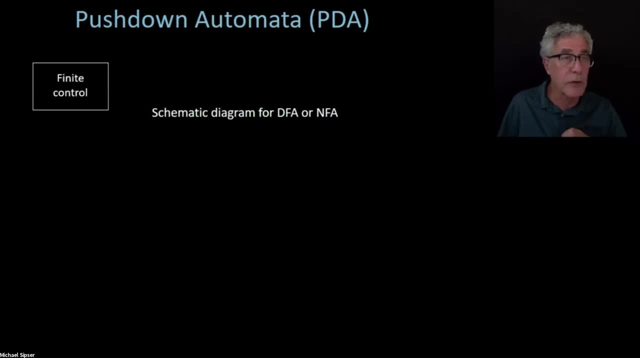 they're really going to be the same from this pictorial point of view. The input is going to be appear on as a string that's written down on what we're calling a tape. Again, this is somewhat of an anachronistic terminology. 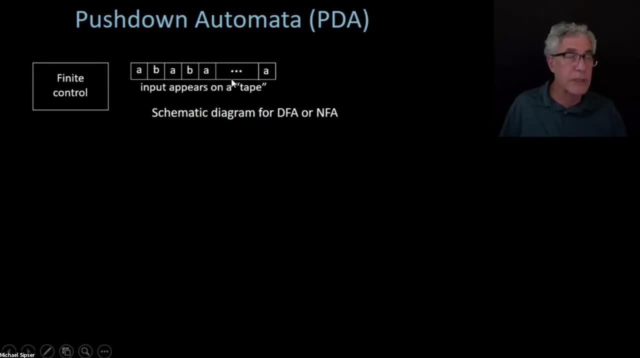 Back in my days people actually did feed their inputs into computers on a tape. sometimes We don't do that so much anymore, but that terminology has stuck and it's going to be persisting later on in the course too, so you might as well get used to it. 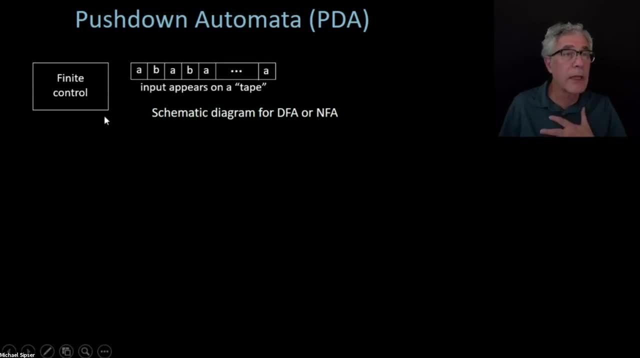 So the input is going to appear on a tape, or sometimes called an input tape, And the way the machine actually will read that input whoops is going to have a head which is going to be starting at the left side and moving from left to right. 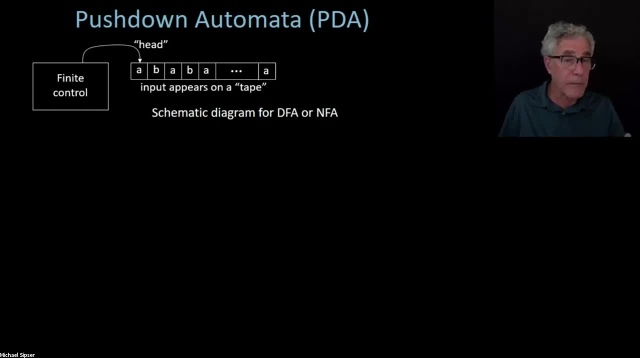 reading the symbols that appear on the input tape, one by one. Okay, so this is our picture of a finite automaton, just redone from last time, just a different way of picturing it. Now that's going to be setting the stage for the picture of a pushdown automaton. 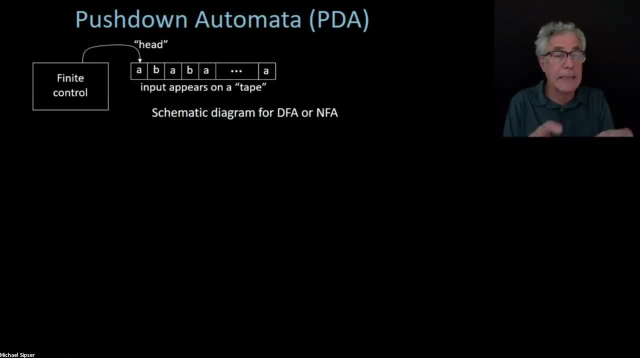 because a pushdown automaton is like a finite automaton, but it has an extra feature, has an extra device attached to it, And that's called a stack. Okay, so here's a schematic diagram for a pushdown automaton And that's going to be a stack. 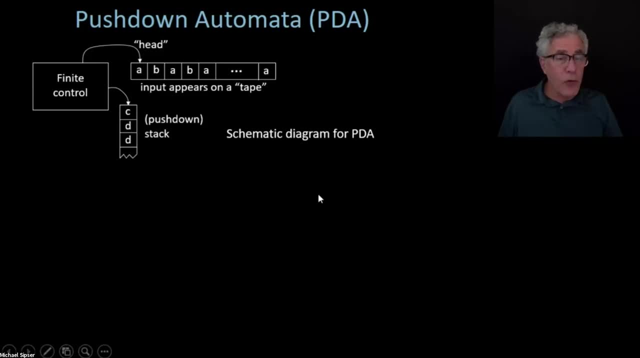 which is going to be basically a form of auxiliary storage. Now, remember, part of the limitation for a finite automaton was that we had a limited amount of memory. Um, so, um, we're not able to do some very simple things like counting because we had a limited memory. 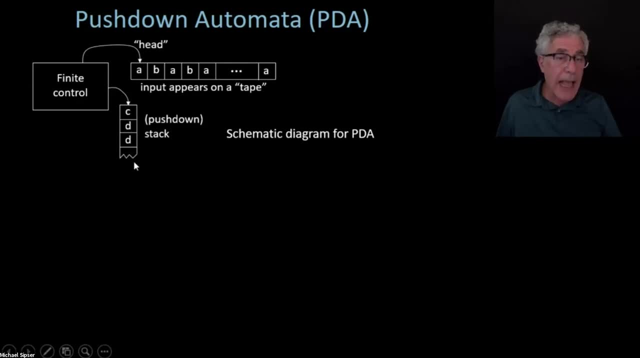 So the pushdown automaton is going to be able to use its stack as a kind of unbounded memory, but in a memory that's very restricted in the way it can be used. So it's unlimited, but still restricted, as we'll see. 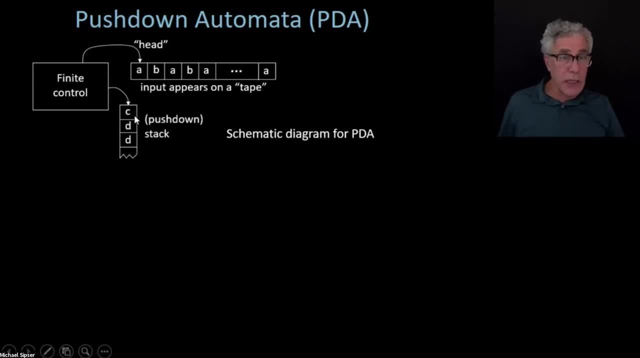 So, uh, the way the pushdown automaton uses um, this extra memory on the, on what we're calling the stack or a pushdown stack, is that you can write symbols um, instead of only reading symbols, but those symbols can only be read at the very. 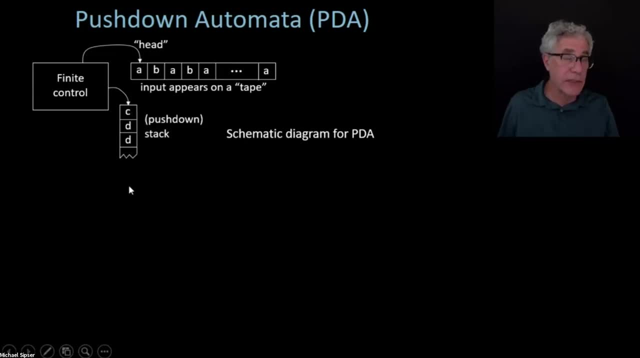 written or read at the very top of this list of symbols, And every time you add a new symbol, the other symbols that are already there get pushed down, hence the name. People also often refer to it as a stack of plates, uh, in a cafeteria. 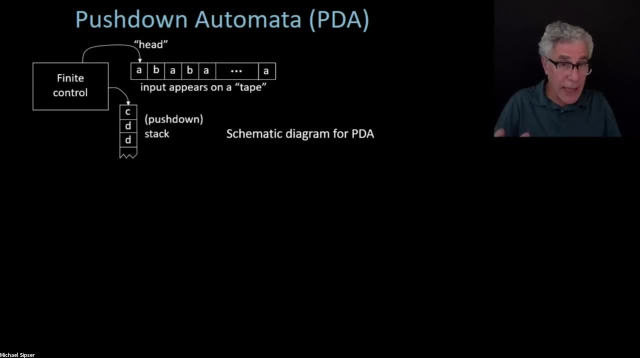 if you've ever seen those things Or you can remember back to the days when we went to cafeteria- uh, which is getting further and further away, But um, uh, if you have a cafeteria, you had a stack of plates. 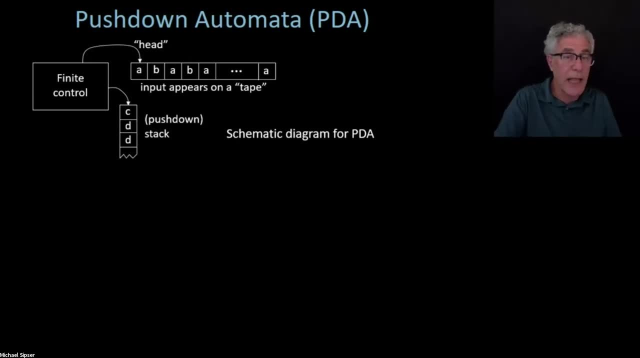 and you know you, as you remove plates from them, there are were on a spring and they kept coming up, or if you add more they would go down, And it's the same idea. Imagine these symbols here are sort of on a um, on a spring. 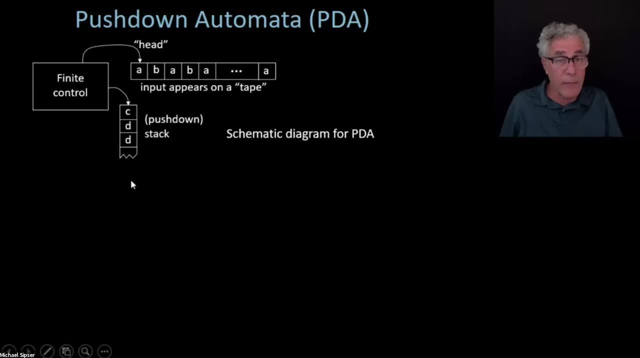 and the more symbols you add, the more they go down. Uh, or if you move them by, read and read them and remove them, then they move back up. Okay, So a push-down automaton operates like a finite, like a non-deterministic, finite automaton. 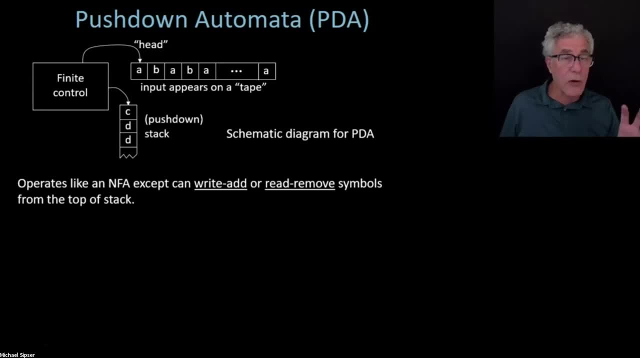 As we'll see, push-down automata for our for us are always going to be allowed to be non-deterministic, So we're not going to be studying the push-down automata that are restricted to be only deterministic. Um, uh, I'll say more about that in a second. 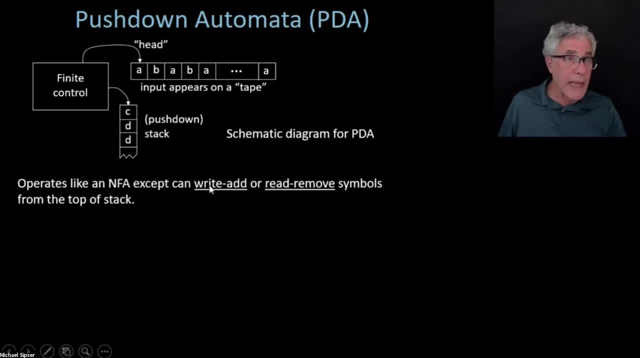 But like they operate like an NFA, except they can write uh or read Symbols from the top of the stack And when they write, they're adding the symbol on pushing down that stack And when they're reading, they're removing symbols from the stack. 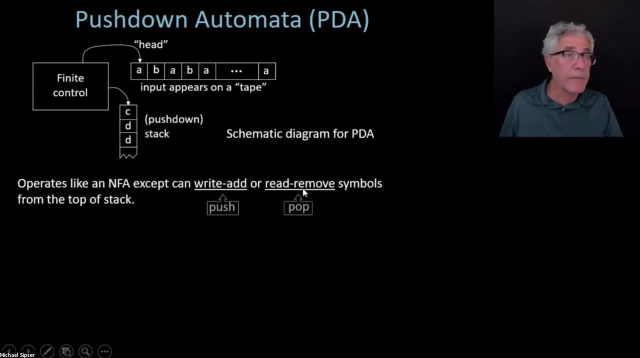 and thereby lifting up the stack. Okay, We give them special names. So those of you who have seen stacks already, this is, you know, I'm sure an old hat for you. Uh, but I'm sure not everyone has has seen stacks before. 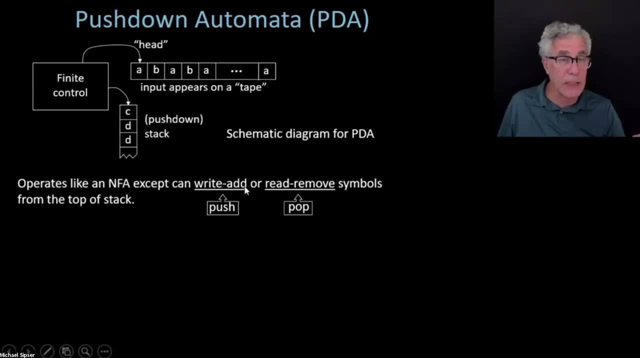 So, uh, the special name for writing onto a stack is called a push automaton. It's an operation so that you're pushing a new symbol down on the top of the stack and it pushes everything down, Whereas when you're reading a symbol and removing it from the top of the stack. 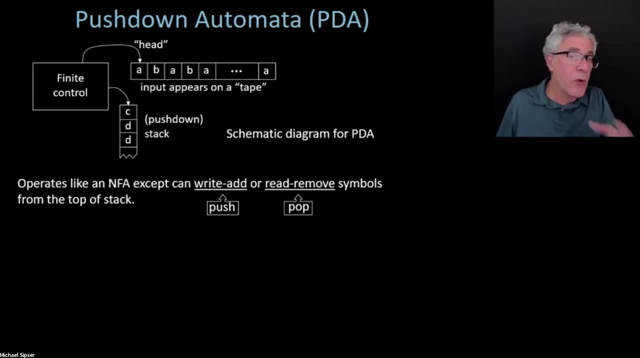 that's called a pop. So that's reading and removing, And we we always think of those as going together. Writing and adding and reading and removing are combined. I mean you might wonder: well, why can't I just read it and leave it alone? 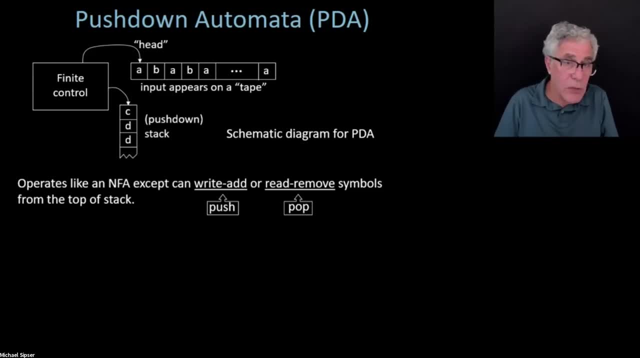 and not just have it remove it. You- uh, no, You can get out of effect by reading it and then, uh, remove it and then putting it back if you really want it to stay there. Um, but the way we're setting it up is that reading comes with removing. 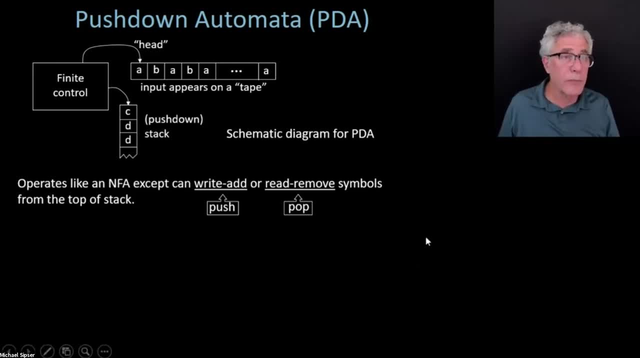 writing comes with adding Okay, and they're called pushing and popping. Okay, so let's do an example. Um, so we have here a push automaton for a language we'll call D. It's a. we've seen that language before. 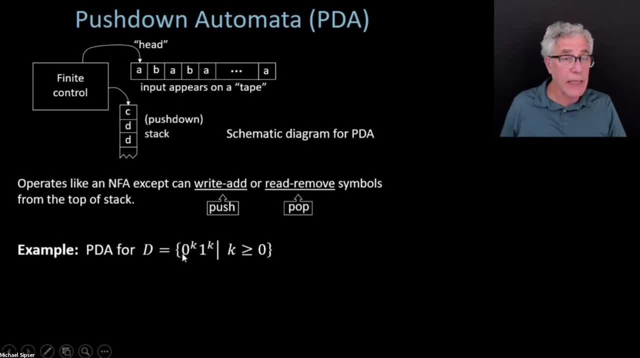 It's this: uh, it was um. actually we used the same uh letter for it. It's strings of zeros followed by ones with the numbers of the same of the two. So zero to the k, one to the k. 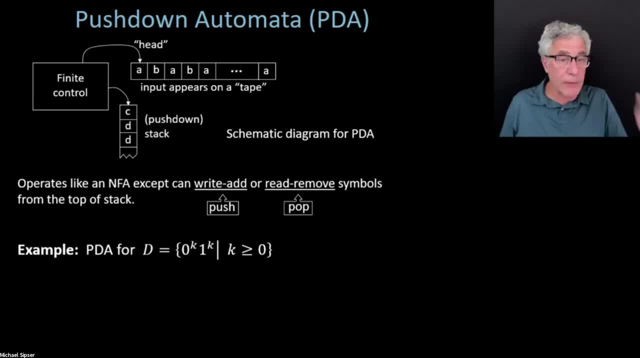 We couldn't do that with a finite automaton. We will be able to do that with a pushdown automaton. Um, and here I uh, um. I thought I wrote down the input here, but okay, So the basic idea is I'm going to give you a, uh, an input now. 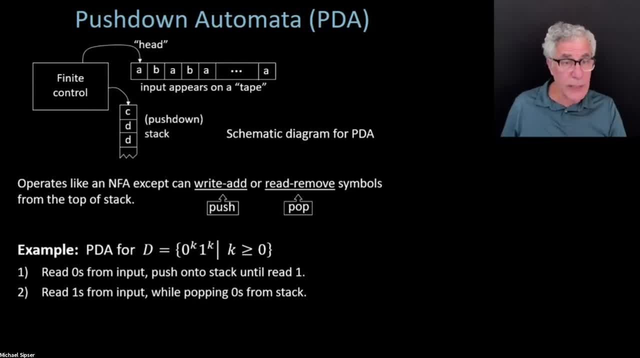 And the pushdown automaton is supposed to test whether that input is in the language, whether it's of this form. Um, now it has the ability to use the stack, because you know it's going to have to count how many zeros it has. 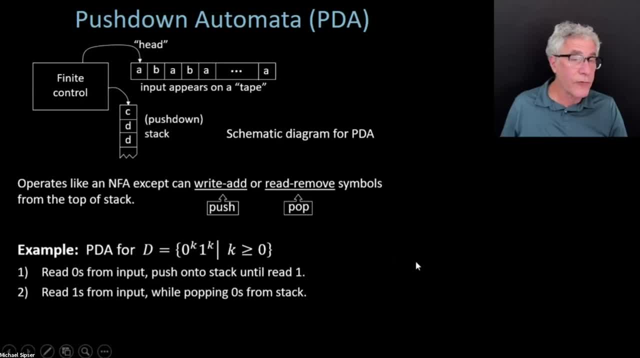 And so the way it's going to do it is that you know, have a bunch of zeros, hopefully, and then a bunch of ones, And you want to see that they're, uh, of the same number. It's going to take the zeros and store them on the stack until it sees a one. 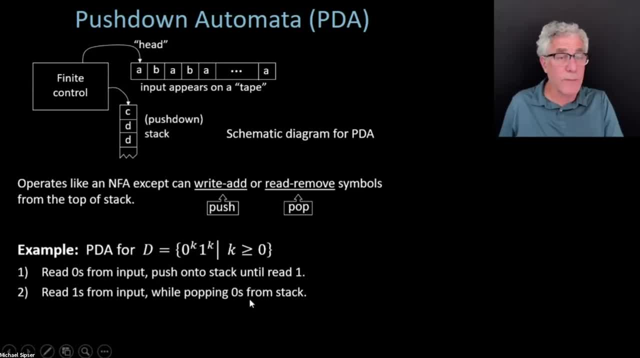 And then one's going to start to read the ones and it's going to remove the zeros, matching them off one to one with the ones that it's seeing. Okay, So, um, you initially first read the zeros and push them onto the stack until you read a one. 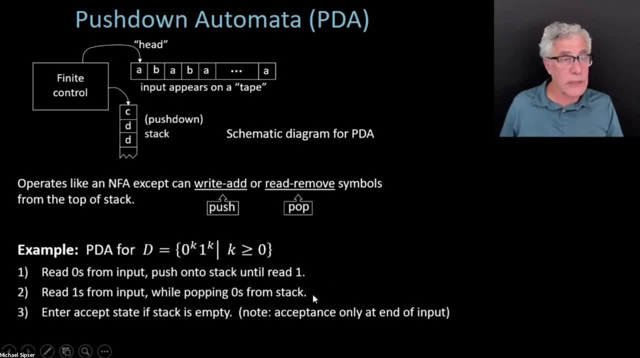 And then you read the ones, uh while uh popping zeros from the stack And you enter the accept state. if the stack is empty, Just like with a finite automaton, the accept- entering the accept state- only counts When you're at the end of the input. 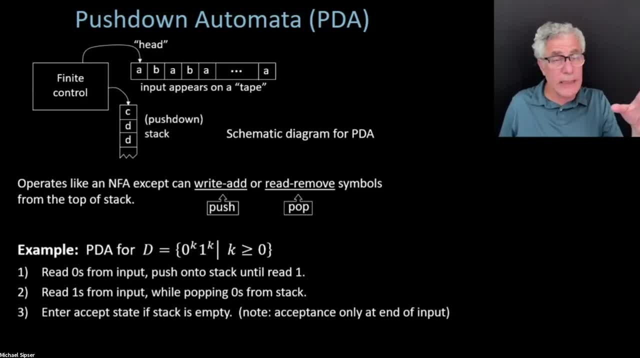 Okay, So um, without even needing to say anything, it's really saying you enter the accept state if the stack is empty at the end of the input string. But that's kind of implicit because it only takes effect at the end of the input string. 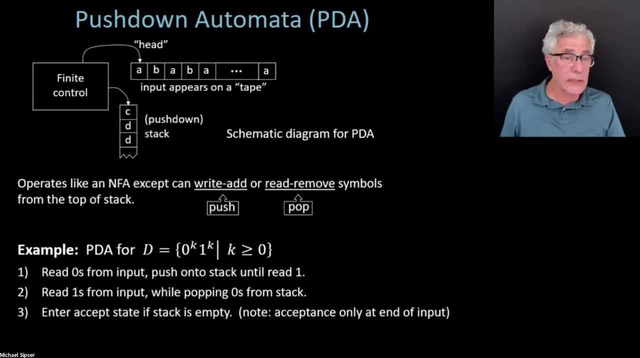 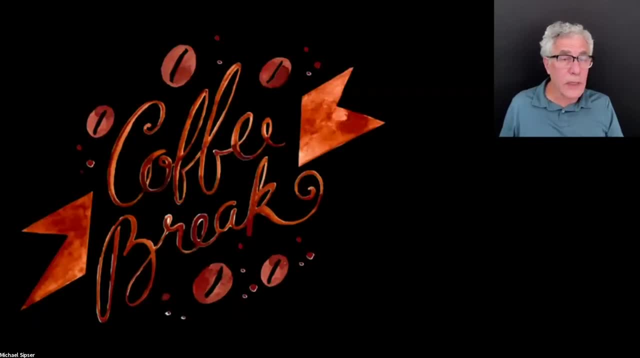 If you enter an accept state along in the middle somewhere, it doesn't matter, It doesn't affect anything. Um, okay, Uh, and with that we're going to take a little break And then we'll be back, uh, shortly to look at pushdown automata again in a more uh, with a more formal definition. 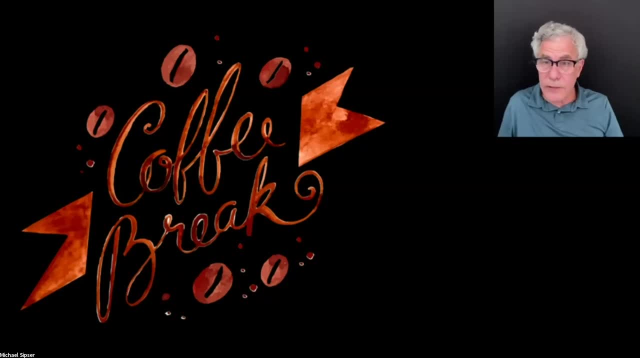 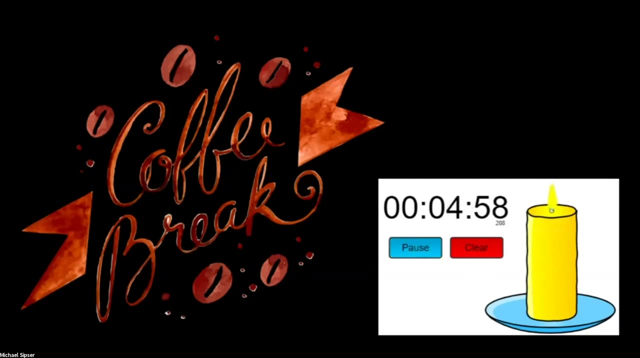 Um, let me put that's going to be five minutes, If I can figure out how to get my timer screen up here. Yes, And we will. uh, when the camera, when the candle burns down to nothing, um, we will return and continue. 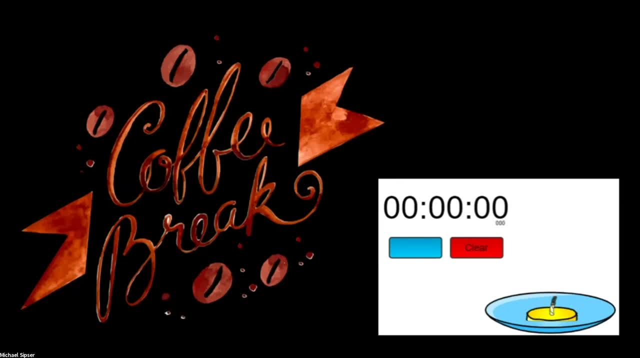 Okay, Our candle has burned down and has gone out. I think I never actually watched to see what would happen at the end. Uh, so, um, we're good to go, Let's continue. Um, uh, good, Let me put myself back in there. 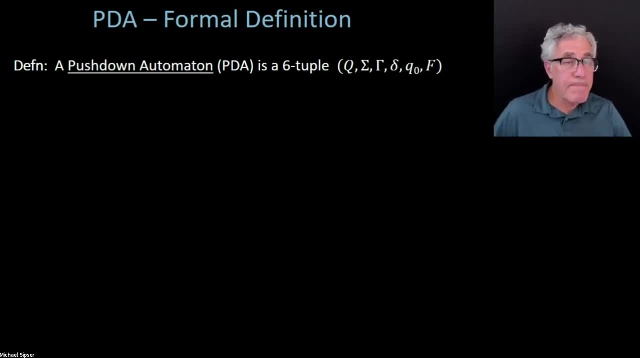 Alrighty, Um, so we were doing pushdown automata, Okay, So we just did that example of zero to the k, one to the k. Now that you have a stack, we can do, uh, all sorts of fancy things that finite automata could not do. um, just with their limited, uh, memory. 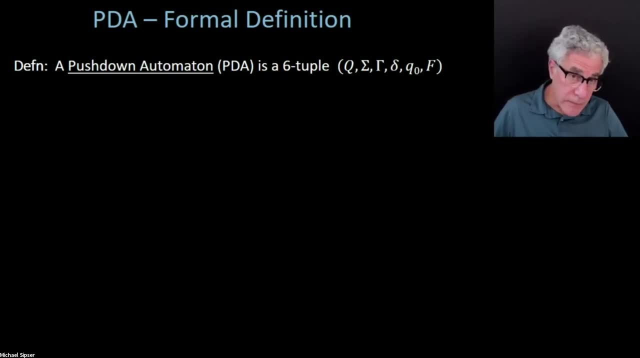 Okay, So let's take a look at how we define pushdown automata. Um, so now, uh, pushdown automata is actually going to be a six tuple, So it's a little bit. We've got some fancier stuff here to deal with. 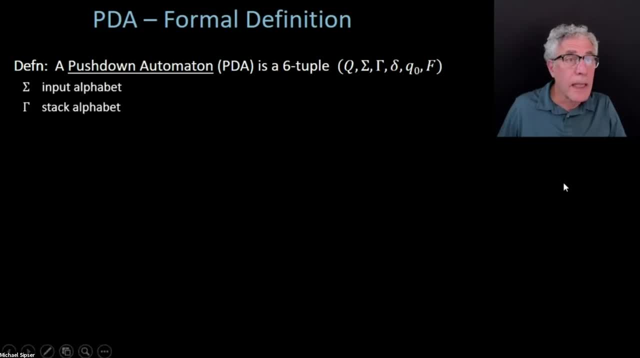 Not too much, but a little bit Um and uh. so it has uh. let's look at these a little bit more carefully, since there's some novelty here. We have the uh input alphabet, just as we had before: uh sigma. 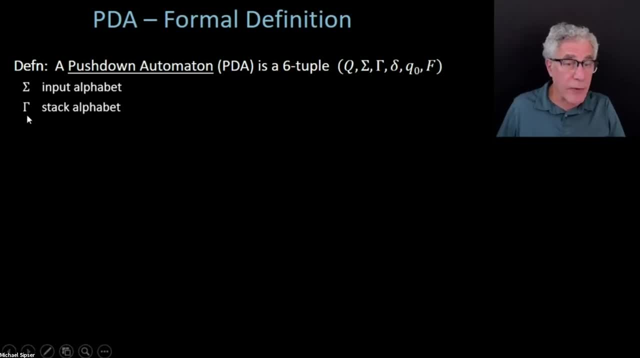 We also have gamma, which is the alphabet for uh using the stack. Now, um, you might ask: why don't we just use the same alphabet? Well, it's really a matter of convenience, um, that we would like to be able to have um, uh, other symbols, that uh could include the input alphabet, but could include other things as well. 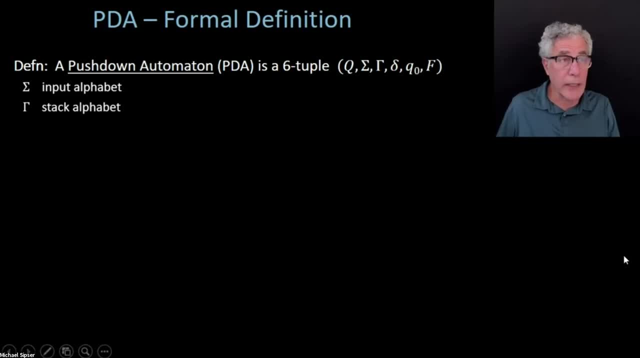 So it just gives you more flexibility in terms of what you're going to be writing on the stack. Um, okay, The transition function more complicated, Uh, so I, I think I don't know if I'm going to even say what the other things are, but you know, these are the accepting states. 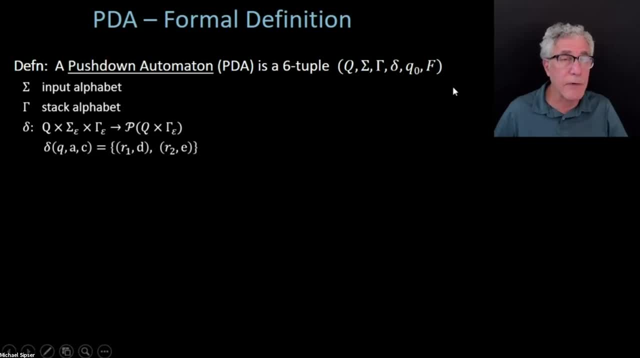 This is the starting state, So that's um The same as before, but the transition function is a is a much, much different animal here, uh, in a pushdown automaton, So let's just try to uh unpack that and understand what it's saying. 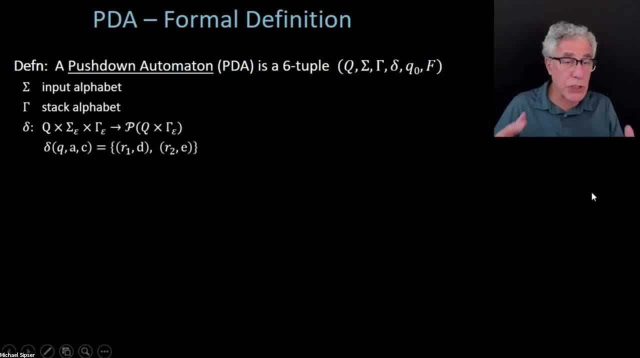 So the transition function tells us how the machine operates, how it goes from state to state, Um, how it's going to read the input, how it reads from the stack and what it might write on the stack too, because that's going to all happen under program control. 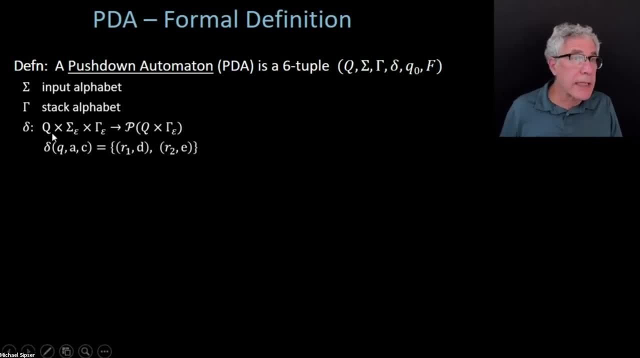 So, um, what this means here is that you know when the machine is in a particular state um reading a particular input symbol. let's ignore the empty string, uh, subscript for the moment. So it's in a particular state reading a particular input symbol and with a certain stack symbol appearing at the top of the stack. 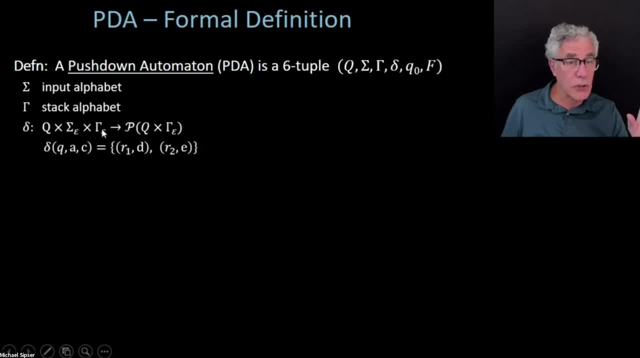 So that's all information that's available, That's available to the controller of this pushdown automaton: The transition function Um, the current state, the next input symbol and the symbol at the top of the stack. And once we have that, we know what new state we can go into and what new symbol we can write on the top of the stack. 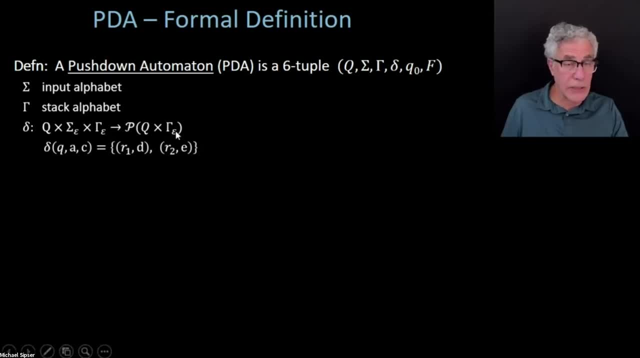 Okay, So that's what the uh, um, right hand symbol does. Okay, So that's what the right hand side of this function specification means. So this is where, uh, kind of the input to the function. This is going to be the output of the function: state entry and new symbol to appear on the stack. 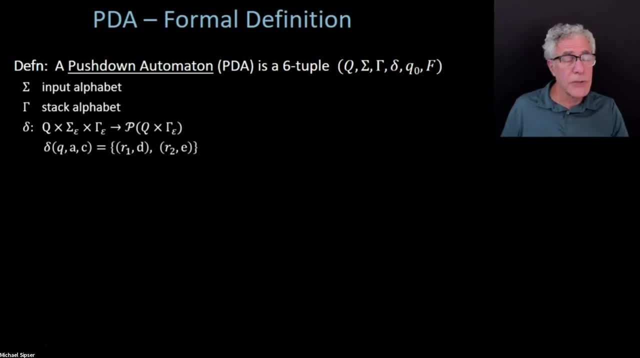 So this is the popping symbol, This is the pushing symbol. So now there are two things that bear explanation here. First of all, now this is: this is a power set, So this is going to be representing, as we did before um, a non-deterministic machine. 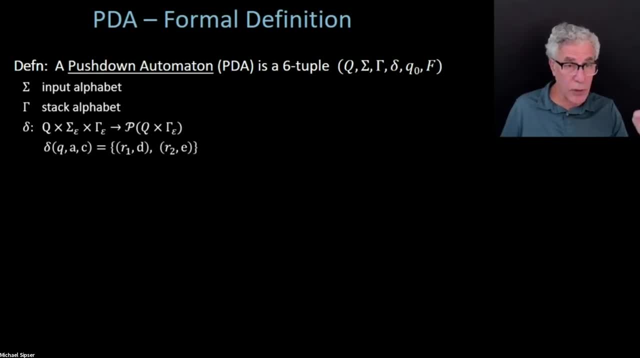 Uh, we may have several possibilities and we're going to represent that as a set of possibilities, uh, for the machine that it could go to at any point. I will give an example of how a pushdown automaton uses its non-determinism in a minute. 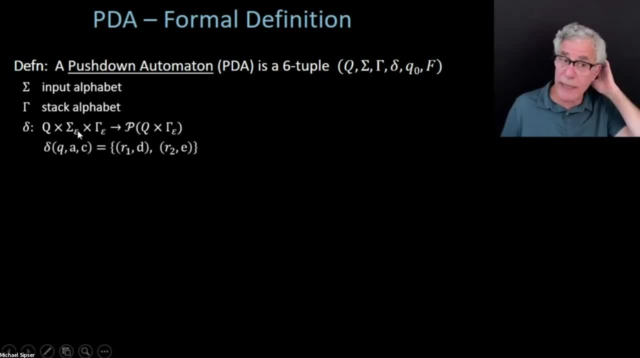 The other thing is: is these epsilons? So we have to understand why they are there And we remember we had them for the NFAs, corresponding to when the NFA had an epsilon in it. The NFA had an epsilon transition, an empty transition. 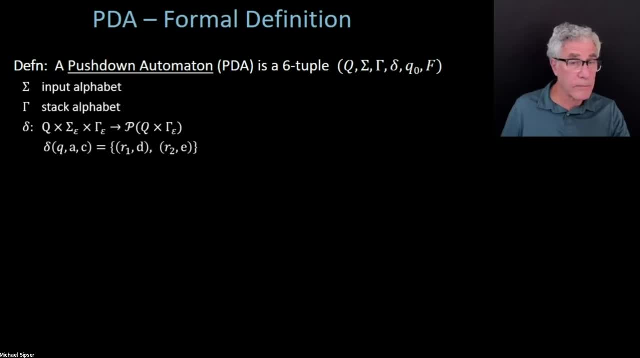 So it could go along that transition without reading any input. So this is going to play the same role here. So if you have um, instead of an input symbol, from sigma appearing in this, um, uh, part of the, you know, uh, for for the, for the transition function. 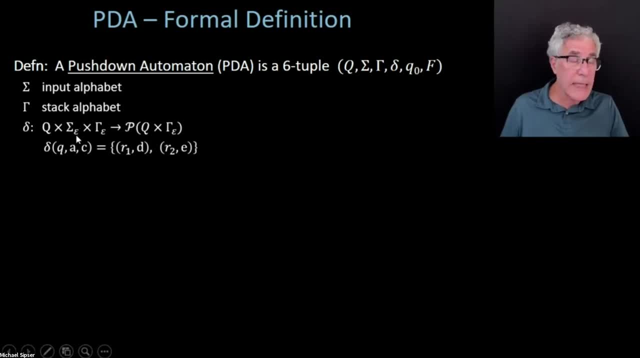 instead you have an, you have an epsilon appearing, That means that the transition, that that move of the machine can happen without reading any input symbol, Just like for the NFAs. Or if you have an epsilon appearing for the stack symbol, that means you can make that transition without reading any stack symbol. 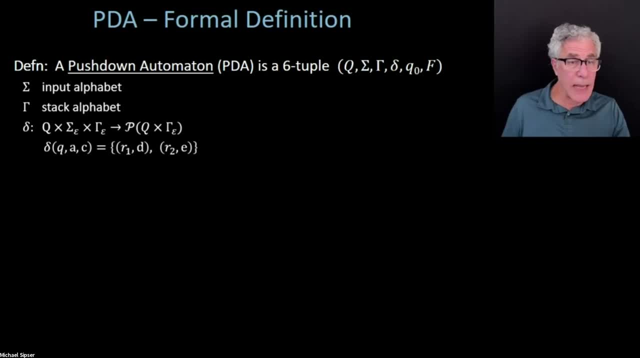 So any whatever is sitting on the top of the stack, it's, it doesn't matter. The machine can make that move, Um, and it won't read anything either. We're not going to pop anything, It's just going to uh, be proceeding without looking at the stack at all. 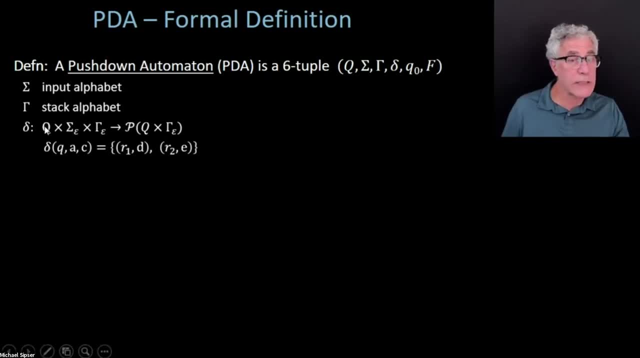 Or it might have both of them, which case it's going to go from one state to another state without looking at the input or at the top of the stack. So, um, that's what the possibility of epsilon means for the um, for the transition function in those in those places. 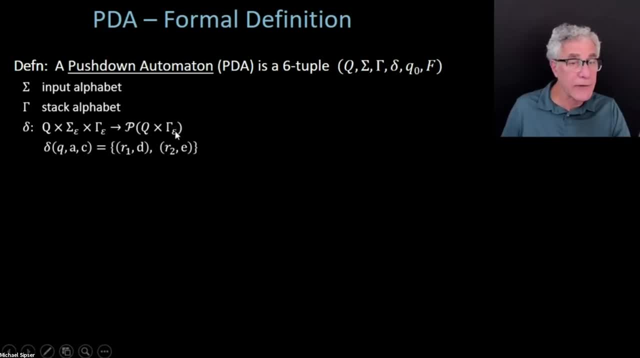 The epsilon appearing over here means something a little different, but very similar. What that means is that, Um, we won't write anything on the top of the stack. That's going to be. uh, we, we will go to a new state, but without doing any writing. 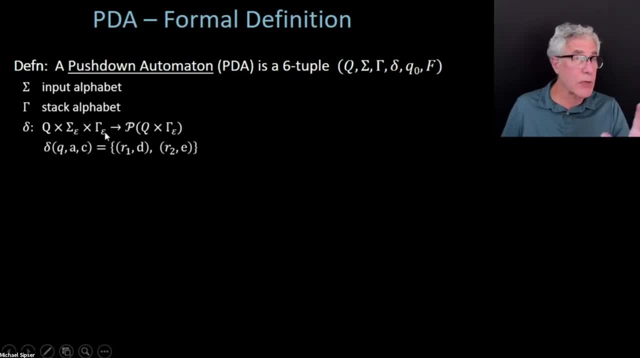 So we'll leave the stack alone. Um, so here means we're not. we're not going to read anything If it's in this position. in this position means we're not going to write anything. Okay, So all of those things are valid and legal from the perspective of, you know, constructing a push-down system. 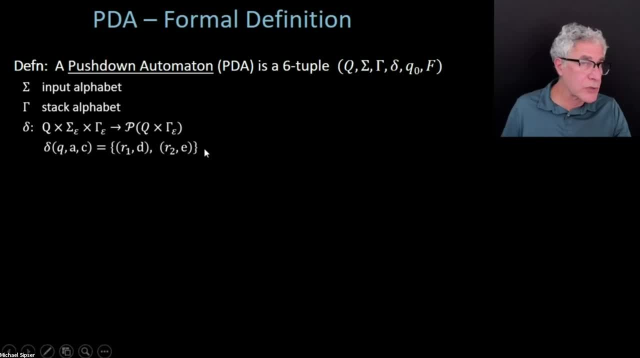 And I've kind of illustrated here, you know, just with a little bit of an example. If you have Delta- that applies to some state Q- reading an input symbol A and popping a C from the top of the stack, Then you might have, let's say in this case, two possibilities that you might end up going to. 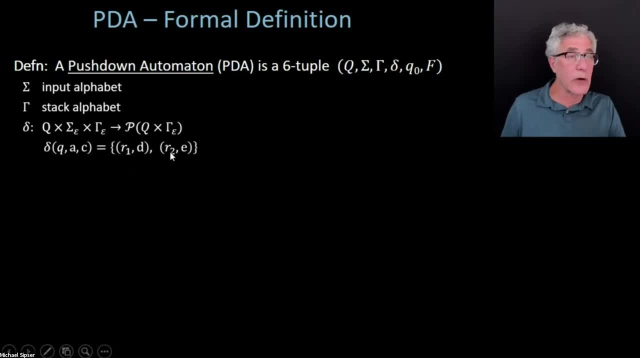 You might end up going to states R1 or to states R2.. And in the former case you'll end up writing a D, pushing a D onto the top of the stack, And in the latter case, you would be pushing an E onto the top of the stack. 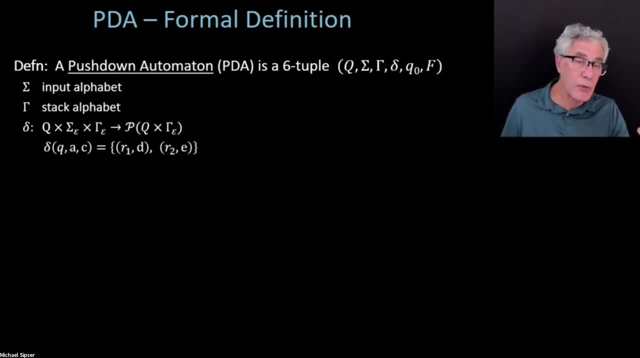 Okay, So this is. I'm trying to help you look at this notation. You can, you know. you know, I hope this is clear to you. Um, I'm sure for some of you it's too slow, but others of you I'm trying to help along. 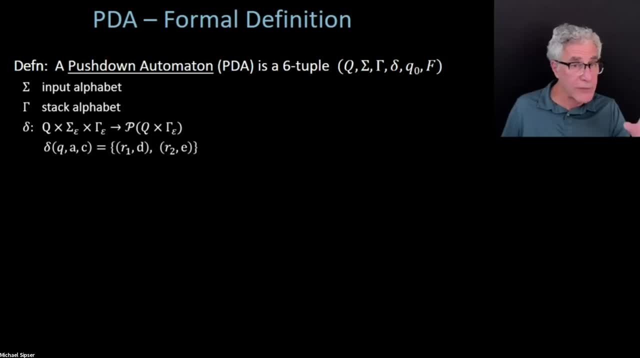 But if you're really struggling with this notation at this point, you know you really have to, going to have to dig in and make sure you follow it. It's only going to get harder from there. It's only going to stop being going over these, these kinds of points. 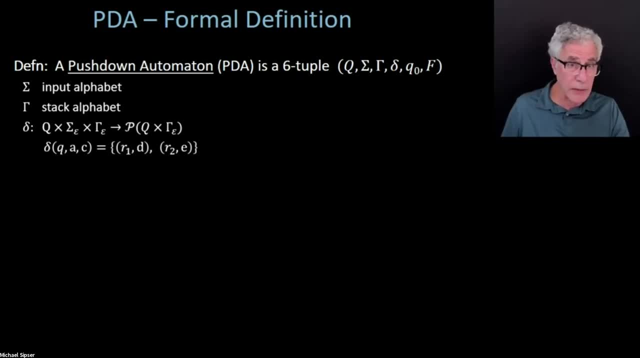 And if you're still struggling, you can't get it. This is not the right class for you. I'll just I'll be honest, Because we're just going to be taken off. like you know, we're going to start to accelerate fairly quickly. 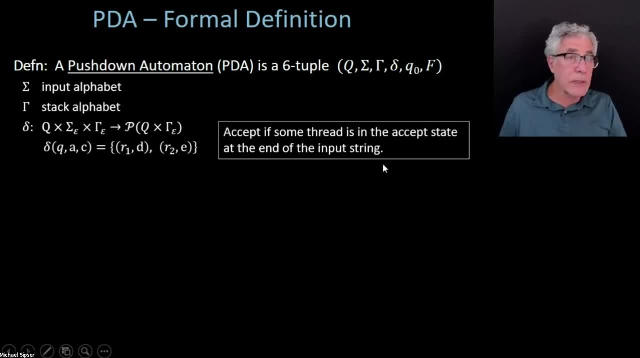 Okay, So it's a non deterministic machine. We accept, like we did before. there might be several different threads of the computation. You're going to end up accepting if some of the threads, or at least one of the threads end up, ends up in an accept state at the end of the input string. 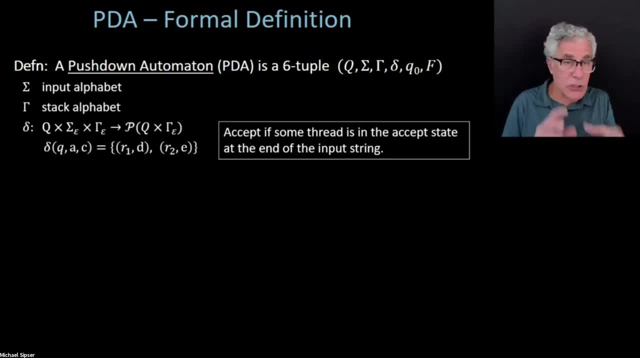 Okay, That's when we machine overall accepts. It's just the way we normally think of non determinism. Again, you can use the models that we had before in terms of guessing or parallelism, whatever works for you, And sometimes different things work in different different at different occasions. 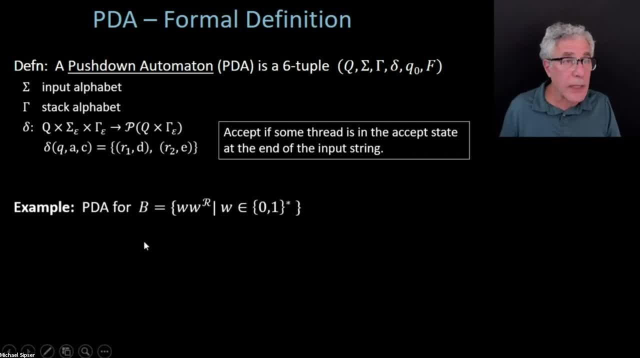 But that's how non determinism works. We'll do an example now. Okay, Here is a push on automaton for a different language we haven't seen before- I don't think- Well, maybe we have- Which is going to be using its non determinism in an essential way. 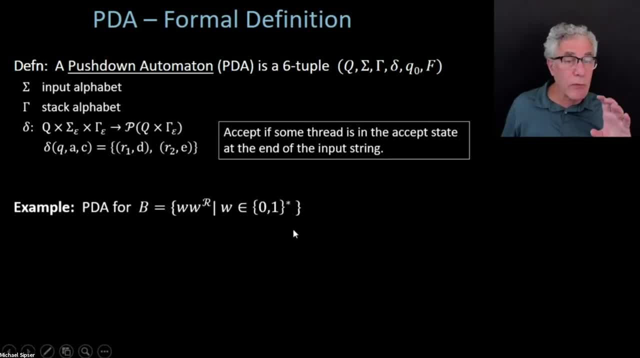 This is a language that is going to where non determinism is going to be critical. Without it, you can't a deterministic push on automaton, which is something, by the way, that people study, And there's a series. 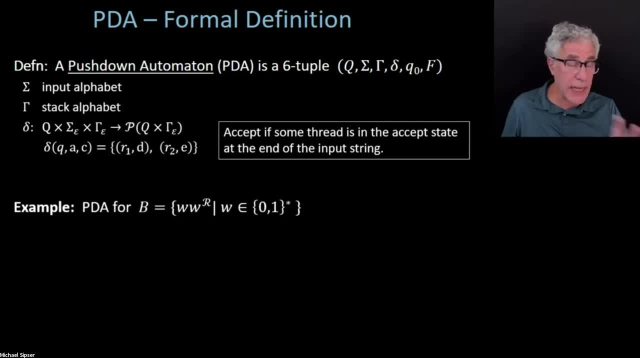 And there's a section of my book about that, section 2.4, because it has relevance to applications. We're not going to address that in this course, So you can just skip section 2.4.. It's pretty technical, I'll have to say. 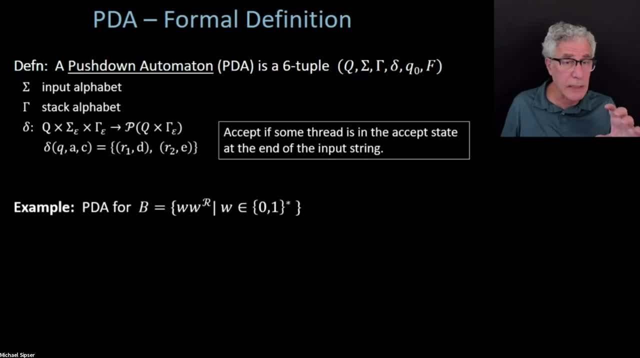 But still quite interesting and beautiful, if you like that stuff. But it's technical, We won't do it. So here is this input string: ww reverse for all possible w's over our alphabet 01.. Okay, And what w reverse, by the way, means is writing w backwards. 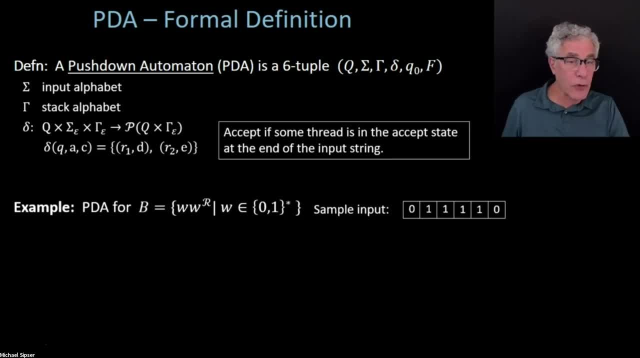 So this is all strings followed by a reversal of the same string. Okay, The string written backwards. Really, you can think of these as you know. so these are strings that well. here's an example: 011110.. The string written backwards. 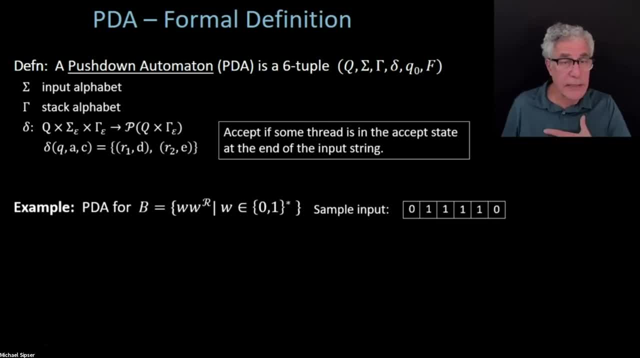 So this is a string in the language Appearing on a tape As I described. Okay, So how is the machine going to recognize this language? It's going to be similar, somewhat similar to before, but with one important difference And, if you imagine, I think again. I like to use this kind of anthropomorphizing these things. 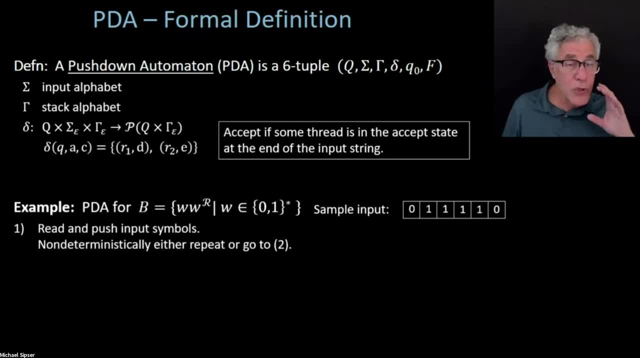 Putting yourself in the place of the machine And thinking how you would do it. So if you imagine getting these symbols one by one, 011.. You don't know what's coming next. as you're getting the symbols, You have to figure out how to match off the second half with the first half. 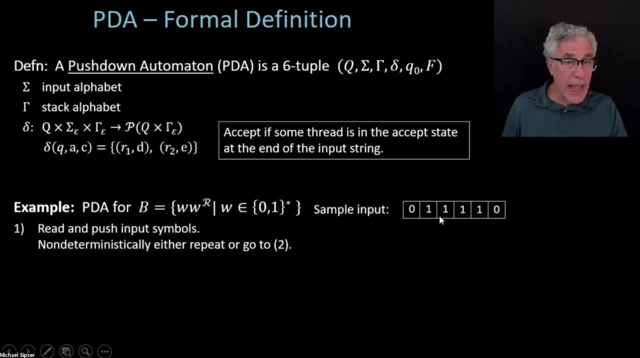 So you're going to put the first half on the stack And then you're going to remove the first half and match it off with the second half. Conveniently, the first half comes out backwards. The stack is a first in, last out kind of thing. 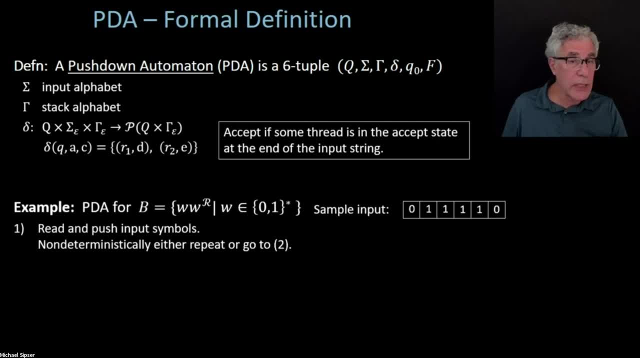 So it comes out in reverse order. So that's perfect for matching. So that's perfect for matching off with the second half. But the tricky part with this language is how do you know when you're at the middle, Because you don't get to see the rest. 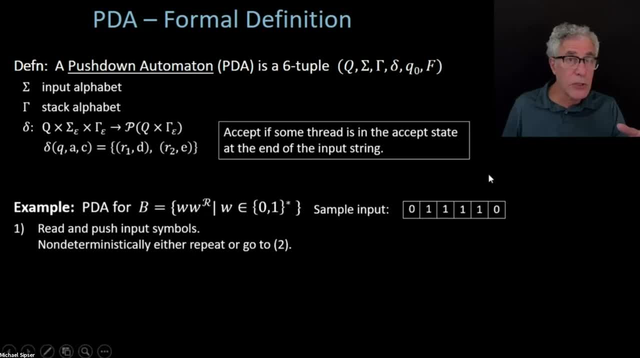 You only get to see what you've seen so far. You don't know what's coming. So you know, when you read that second one, at this point you read 011.. Now you're reading that second one. You don't know that perhaps there's just going to be a 0 following that and it's going to be all. 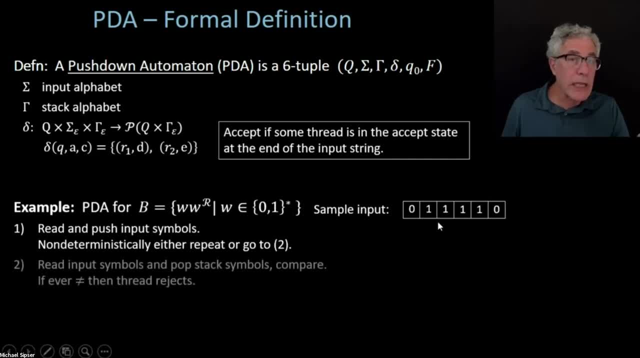 So maybe you should be deciding that this point here that I've marked is the midpoint And you put 01 on the tape and then start popping the second one and matching it off with the first one. That would be a tempting thing to do. 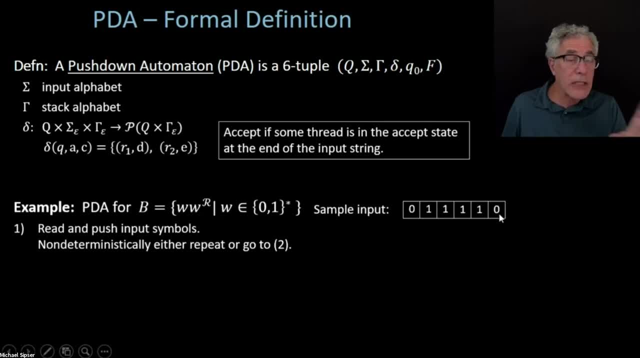 But you just don't know, And that's where the nondeterminism is going to be essential. So let me write down more of this. So what you're going to do is you're going to read and push input symbols, but nondeterministically, guessing that you're at the middle. 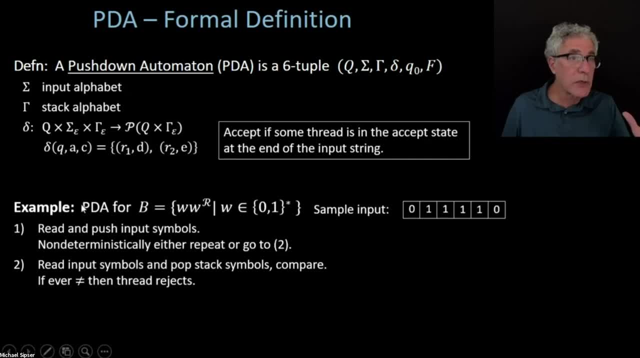 So you're going to nondeterministically either repeat that and continue to read and push symbols onto the stack, Or you're going to go to 2, deciding that or guessing that. you're at the midpoint And now it's time to start reading and popping instead of reading and pushing. 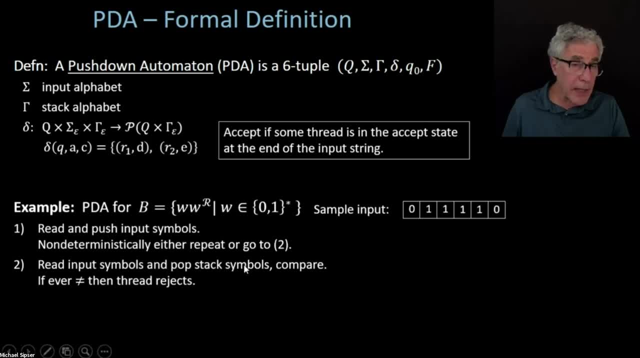 Okay, So you're going to read input symbols and popping the stack symbols, comparing the two, The symbols that you're reading with the symbols you're removing from the stack. If they ever disagree, then this thread of the nondeterminism rejects. 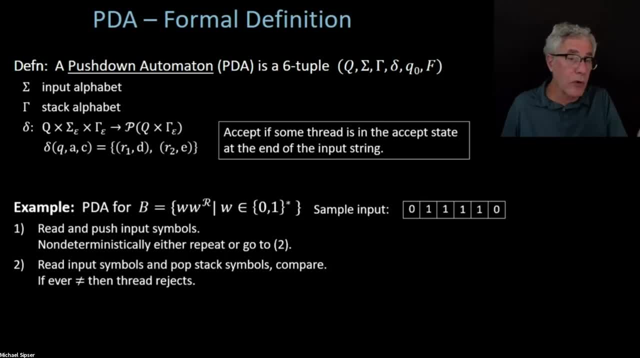 Because either the input is not in the language or at least you've made a wrong choice as to where the midpoint is, And then you're going to enter the accept state if the stack is empty And ignore this part, for the moment, of this software reference. 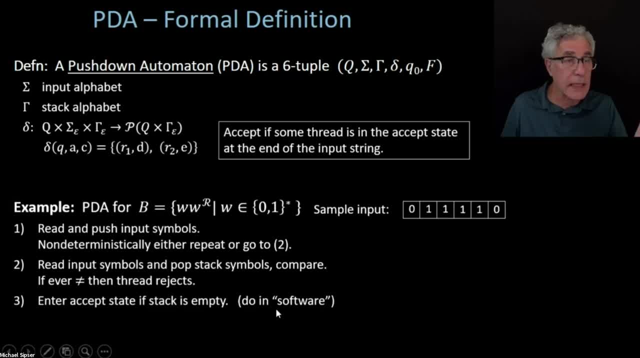 Let's just- I'll speak to that in a second, But I just want to make sure we understand that at an intuitive level- how this machine is using its nondeterminism to recognize this language, Because the nondeterminism is critical and it's important that you understand it. 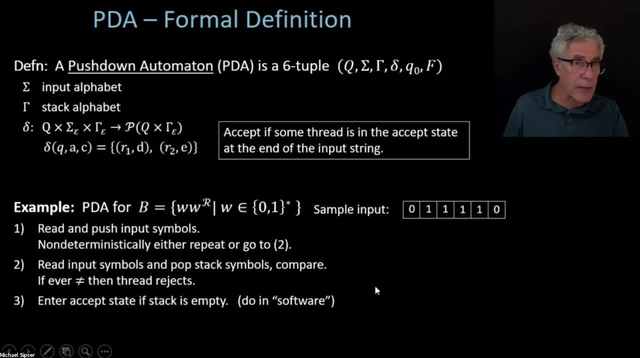 So let me just make some side comments and then we'll come back to this software remark. So first of all, one question that comes up a lot. I'm not paying attention to the chat here, Sorry, So if you're not getting answers from me, try the TAs. 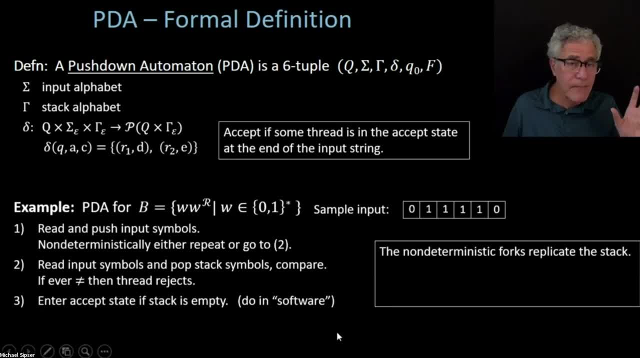 But one of the questions that comes up a lot when they're thinking about nondeterminism for pushdown automata is: what happens to the stack? The stack gets replicated In the nondeterminism every time the machine forks, just like everything else gets replicated. 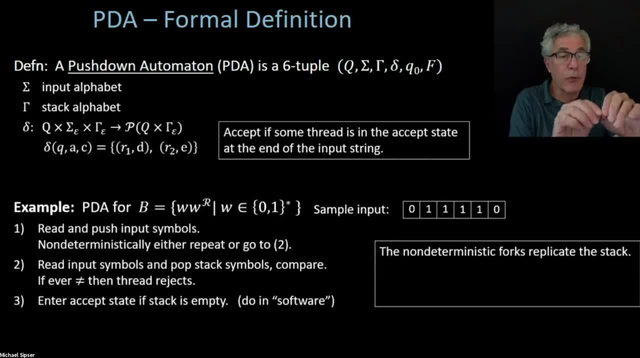 So an entire. every time there's a fork in the nondeterminism and the machine branches into multiple possibilities, the entire machine replicates The current state, the current position of the head, the stack and its contents. all of that gets replicated. 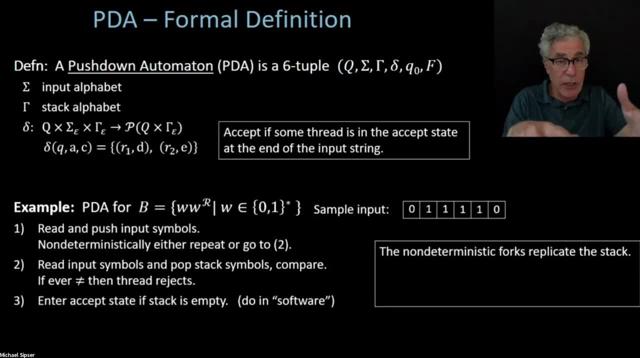 And the two sides of the, the two branches or the two sides of the fork, each go on independently in their merry way, doing their own thing independently, And then, if any one of them accepts, that's the only way, there's sort of a kind of a communication. 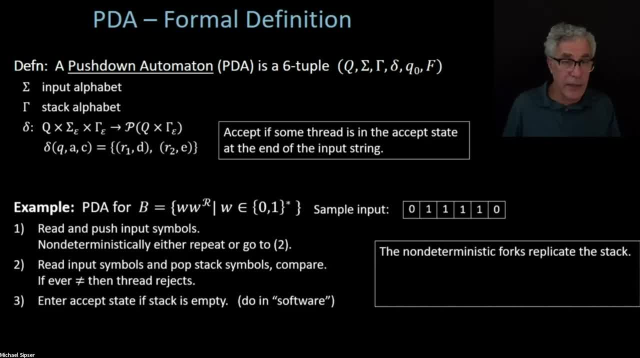 because the one that accepts raises the flag and then the overall machine is set to accept. So the nondeterminism forks replicate the stack. I'm saying it just want to make sure you got that, And then this language requires nondeterminism. that I said earlier. 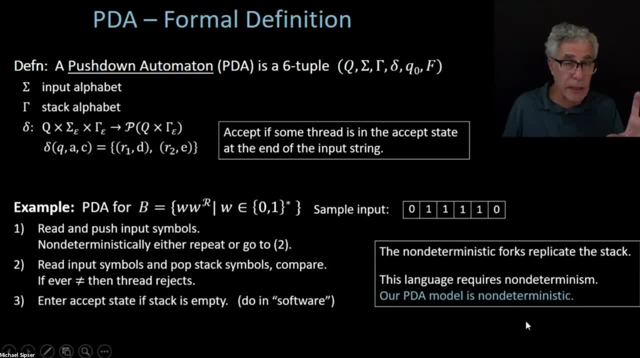 So our PDA pushdown automata is going to be nondeterministic. I mean, you might have examples which are deterministic, but the model is going to always allow nondeterminism. OK, what's this bit about the software? 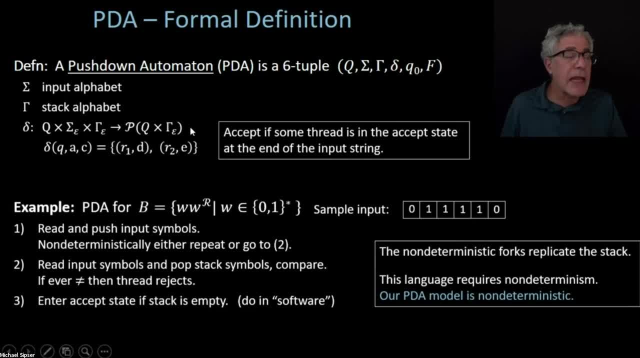 So if you look at this formal definition here, it doesn't have anywhere in it the ability to test if the stack is empty. That's not part of the hardware specification, at least as we are describing it, for a pushdown automaton. You can imagine somebody else describes pushdown automata in some other way. 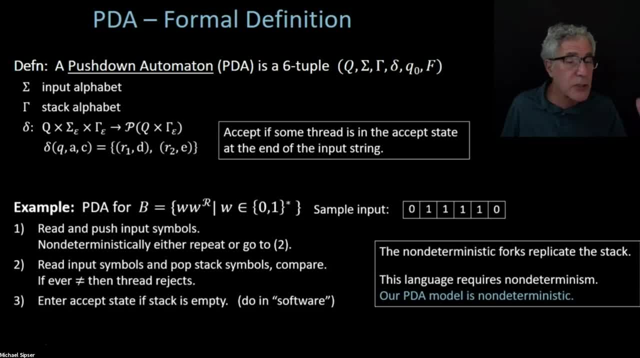 which gives that as a primitive. We're not going to do that. Why? Because we don't need a primitive for that. You can get the effect of testing if there's an empty stack, even if you don't have that as a primitive for the machine. 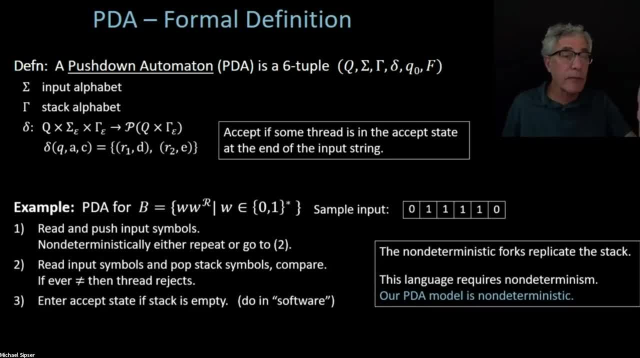 Because what you could do is you could start the machine off when it, at the very first thing it does is it writes a special symbol to mark the bottom, what's going to eventually be the bottom of the stack. There's going to be some special symbol, maybe a dollar sign symbol. 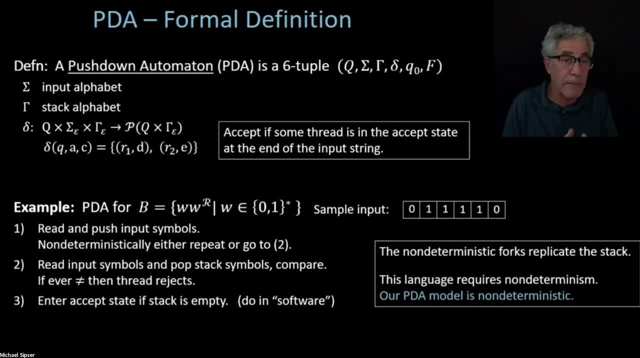 That's the very first thing that the machine does, And then it proceeds as before, And if it ever sees that dollar sign symbol again, it knows the stack is effectively empty. OK, so you can get the effect of testing for the stack being empty. 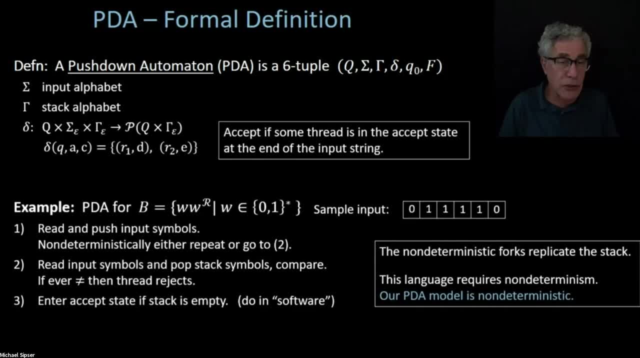 even if you don't have a primitive for that, And we're not going to actually fuss about details like that. So you can use when you're writing your homework sets. you can just use the assumption that you can test for empty stack. 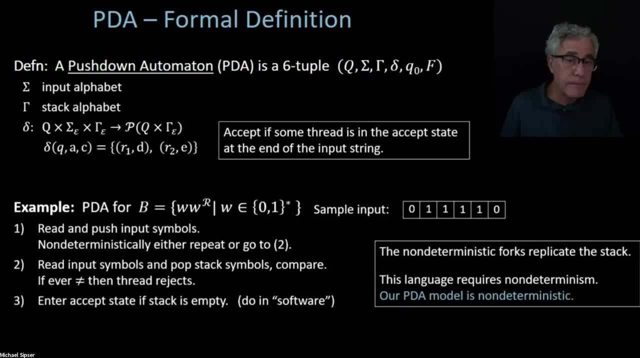 which is what I'm going to do myself. OK, so let's continue on. All right, so yeah, So now what we're going to do? we're going to prove our one. So far, we really haven't proved anything. 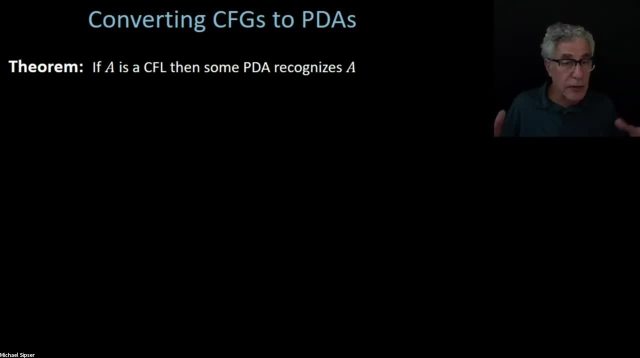 We've just given some definitions and some examples Today. now we're going to come to our big theorem, which actually is important and has some meat to it, And that is: how do we convert? You know, I claim that to put. 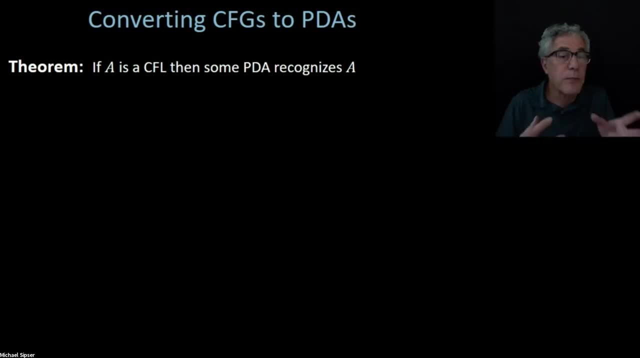 context-free grammars and pushdown automata are equivalent. Well, we're going to prove that equivalence in one direction, converting the grammars to pushdown automata. OK, so let me show you how that goes. In some ways it's a nice proof, not super complicated. 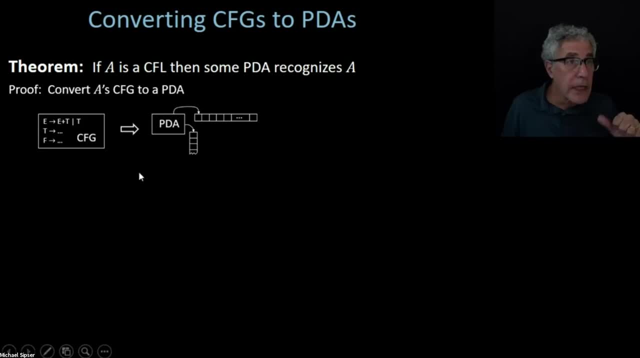 but it has some meat to it. So if I give you a grammar here, what I'm going to tell you how to do is convert that grammar into pushdown automaton, which does the same language. OK, so if you're checked out for a minute, 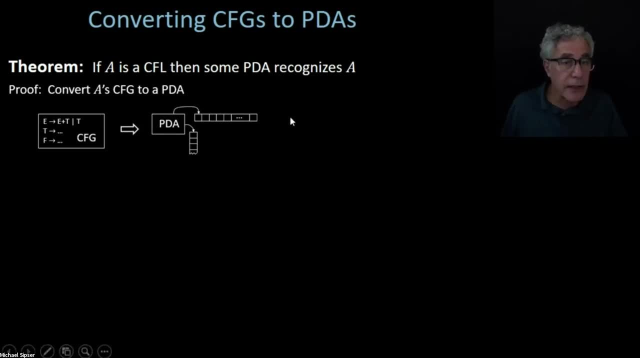 please come back, because we're sort of starting this topic now. You can think a bit about this. Good reentry point if you have sort of been doing something else which I can't tell, Good thing, All right. so converting a given grammar to a pushdown automaton. 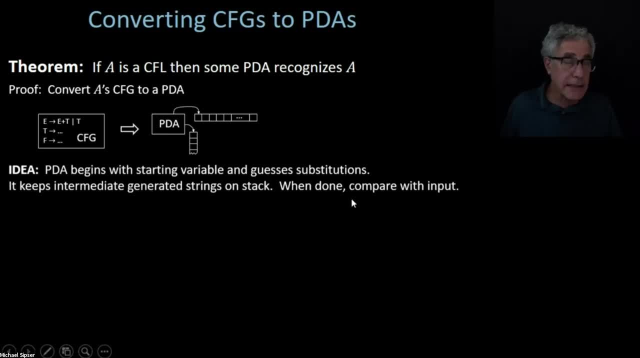 How is that going to work? So the idea is OK. Actually, before I tell you the idea, let's just think about it together. Again. I like to think about the pushdown automaton. building a pushdown automaton, the way you would do it. 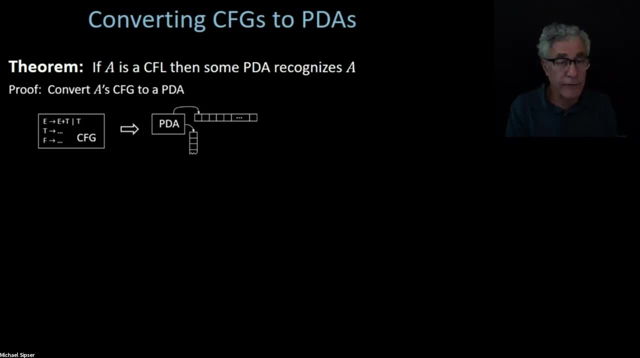 So a grammar is a generation device. It generates strings, A pushdown automaton or thinking about it as you. you're a recognizer, You're given an input and you want to know: is it in the language? So you want to know, is it possible for that grammar? 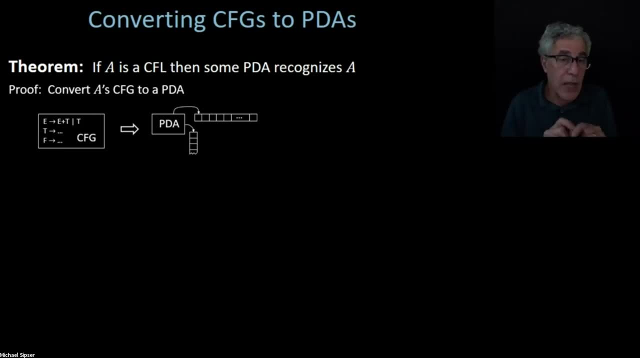 to generate that input you're given. So how are you going to do that And how are you going to test if the input is in the language of the grammar? Well, the thing that you would naturally do is you say: well, can I derive that string using the rules of the grammar? 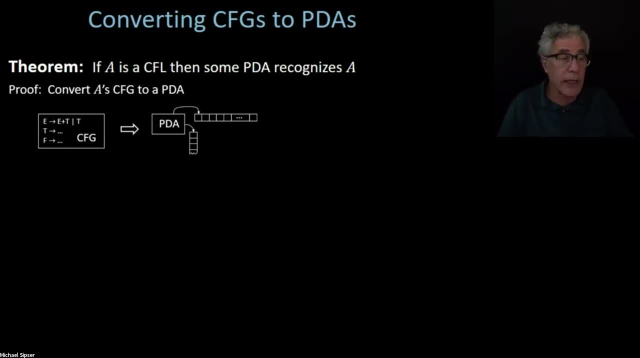 Let me start with the start string and try to do substitutions and see if I get the string I'm given. And if I can get it then I know it's in the language. That's a natural thing to do. You're just going to try to do the substitutions. 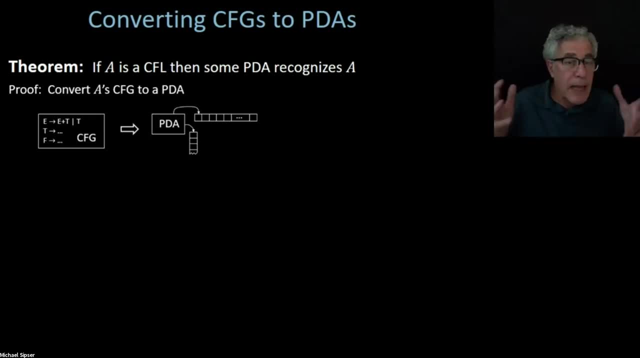 see if you can get to the string. Now the thing is there might be many different substitutions that you could make, And that seems like a really challenging, hard thing to figure out which substitutions to use among the many possibilities. That's where non-determinism is going to come in. 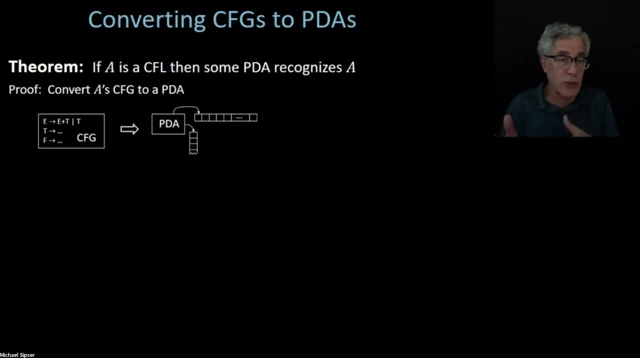 Because you can think of yourself as guessing which substitutions to make and you're always going to make the right guess. So the choices of which substitutions to make, that's not going to be a problem for you. That's going to be managed by the non-determinist. 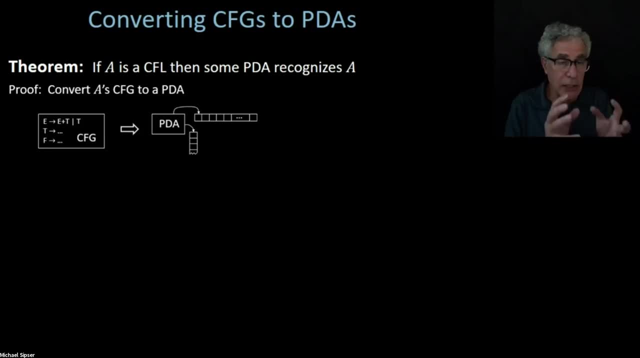 So imagine you're always going to make the right substitution. But now the challenge is: how do you keep track of the intermediate results, as you're doing those substitutions And that's where the stack is going to come in, And then it's going to write down those intermediate results. 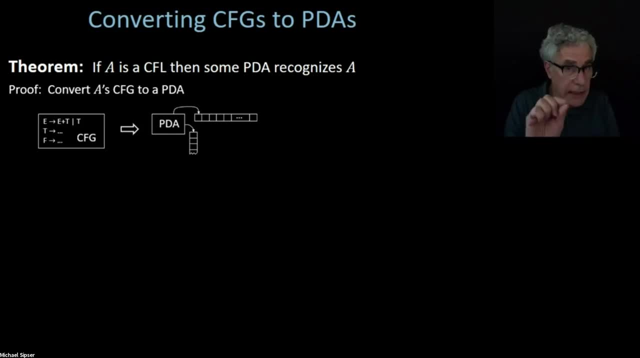 on the stack. But even there there's a subtlety That's an important subtlety that you have to look at. So let's try pulling that together so far before I get to that subtlety. So, as I mentioned, the pushdown automaton. 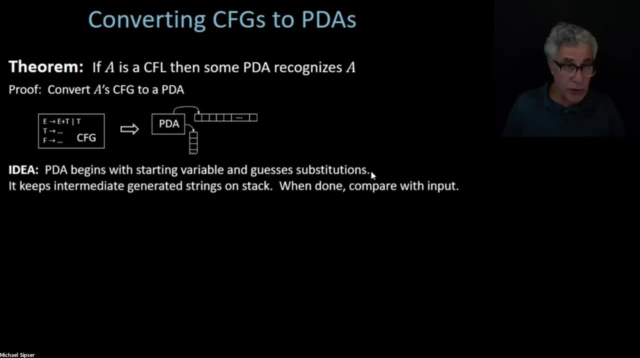 is going to start out with a starting variable and is going to be guessing the substitutions to make And it's going to keep the intermediate results on the stack When it's done doing all the substitutions and it has only terminal strings on the stack. 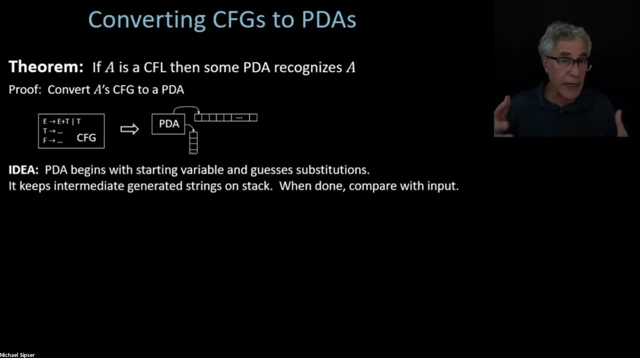 it can compare it with the input and see if it got the right thing, so if it made all the right guesses. So you think of it as guessing, doing the right guesses, But in the end you have to check to make sure that you did all the right thing and you accept. 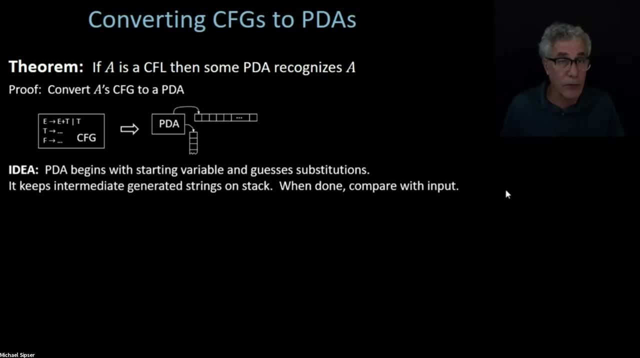 when things have matched up and you made all the right guesses. So in the end you have to check that you actually got that input From doing those substitutions. OK, so let's try to see this operating in action And then you'll see the subtlety, the delicacy. 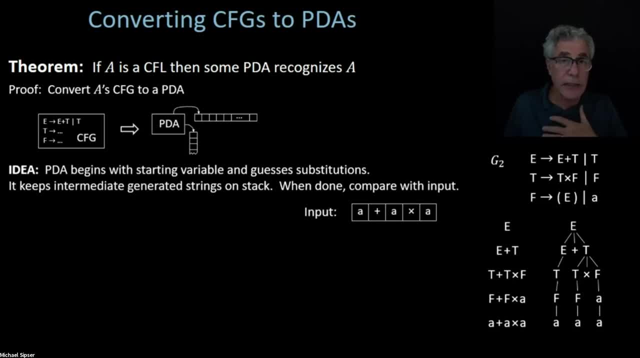 a problem that's going to arise. Hopefully you're following, at least in part, what I'm just saying so far. OK, so here is the input. We do know that that's an input in the language of the. we've been seeing this example multiple times. 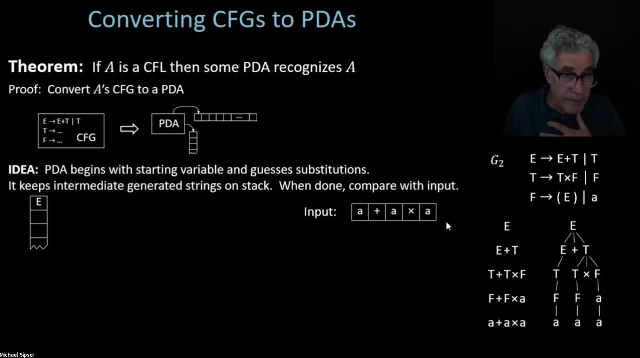 So here is the input appearing on the input tape: a plus a times a. Now the push on automaton is supposed to be accepting that input because it's in the language of the grammar. OK, so it's going to operate by first writing to start off. 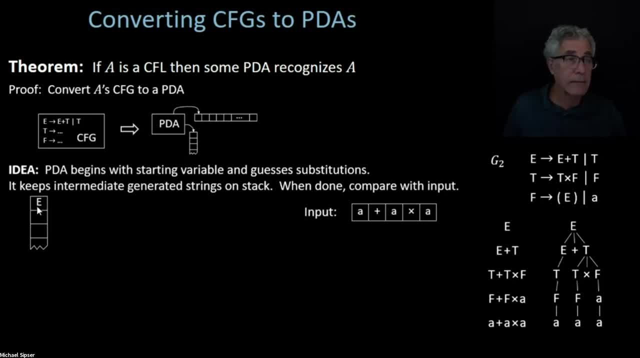 the starting variable on the stack and then doing the substitutions as we're going along. OK, so we're going to substitute: We e goes to e plus t, So we do that first substitution And then we do the next substitution here the e. 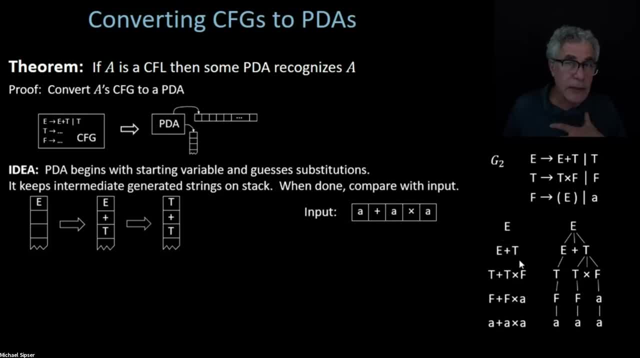 So if you're looking at this tree here, this is the right tree for that input. So we substitute e by t. So far, so good. The automaton can make that substitution. Then the next substitution is going to be a little. 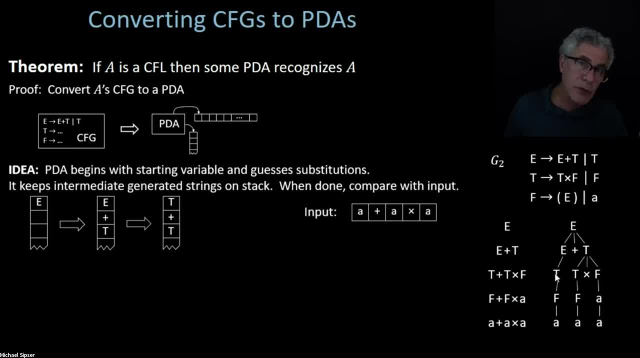 So we're at e plus t, We substitute. here We've got t plus t And now we're going to substitute the t times f, which is this t over here. We want to substitute that And that appears as t times f now on the stack. 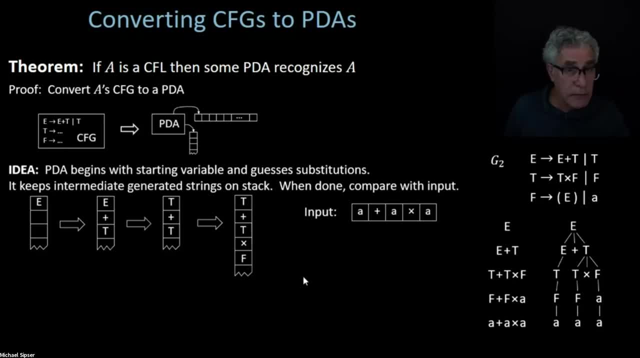 Now, if you're following me, you should be suddenly getting nervous because we just cheated. It's OK Doing these replacements at the very top of the stack, because the pushdown automaton has access to the top. That's how stacks work. 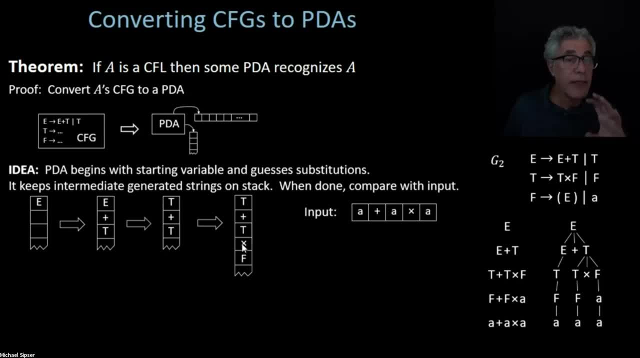 But it does not have access deep down within the stack. That is not how stacks work, So that's cheating. But ignoring the cheating for the minute, if you could replace those, do those substitutions deep down within the stack, this would all work. 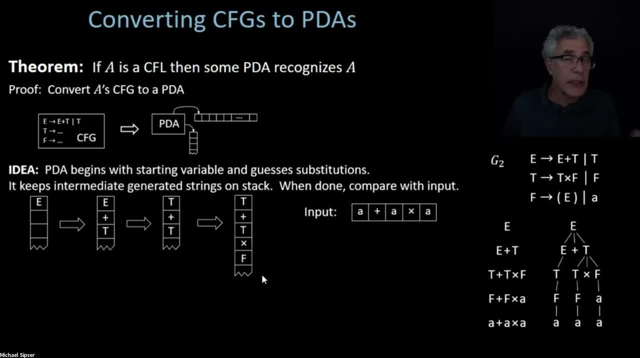 We would be good. You would do the substitutions one after another until you ended up with no variables. And then you have the string here And you're going to match it off and compare it with the input. It's all done in the right way so that the things are. 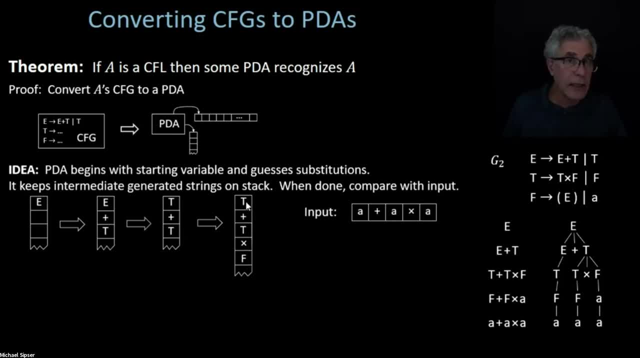 in the right order. So after all the substitutions, you'd have a plus a times a sitting here on the stack. You match, You compare that with the input, It's going to match up And you'll end up accepting All good. 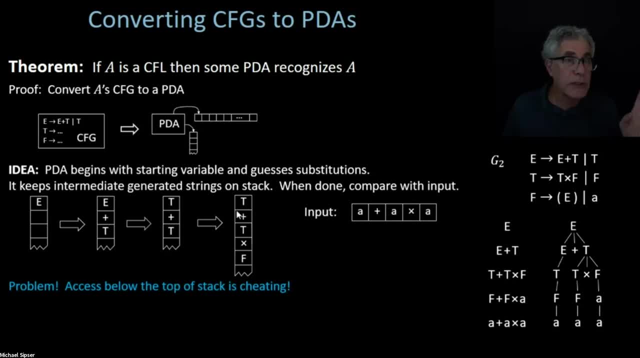 So how do we deal with that problem here? Problem: access below the top of stack is cheating. What are we going to do instead? So the idea is actually pretty simple. Well, if you've understood what I've said so far, fixing that is actually not too bad. 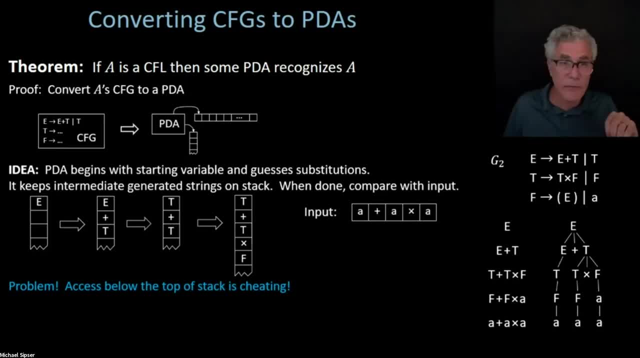 Sort of fading out here, Put some more light on my image. So how do we do that? How do we get the effect? How do we get the effect of the access below the top of the stack? And the way we're going to do that is by making the 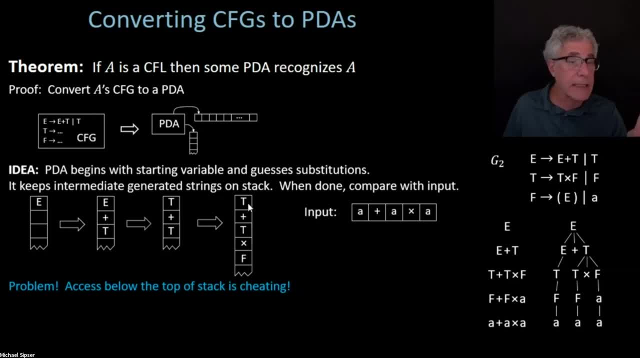 what we're going to do. we're only going to do substitutions that we can make at the top of the stack. So whenever there's a variable at the top of the stack, we're going to do the substitution, Because the top we can't access. 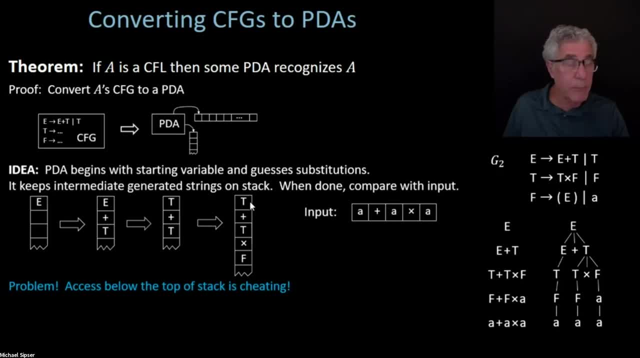 Now, what happens if we have a terminal symbol sitting at the top, blocking our way from accessing variables below? Well, actually that's an easy question. That's an easy case to handle, Because if we have a terminal symbol sitting at the top, 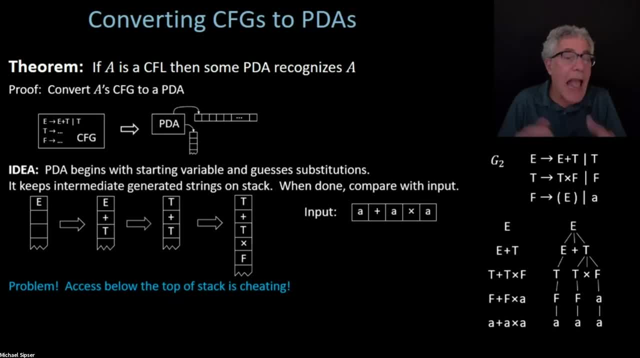 they're never going to change anyway, So you might as well match them with the input at that time. So when you have a terminal sitting at the top, we'll just read another input symbol and match it off there And we just keep reading the terminal symbols off. 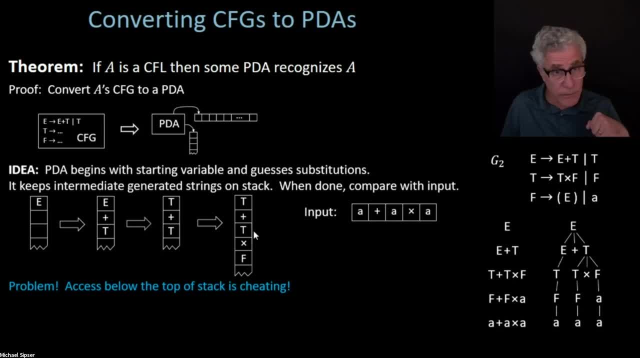 until we have a variable sitting on the top. Then we do a substitution And we keep substituting variables at the top of the terminal. Then we read it, Then we compare it with the input And in so doing we will end up getting the same effect. 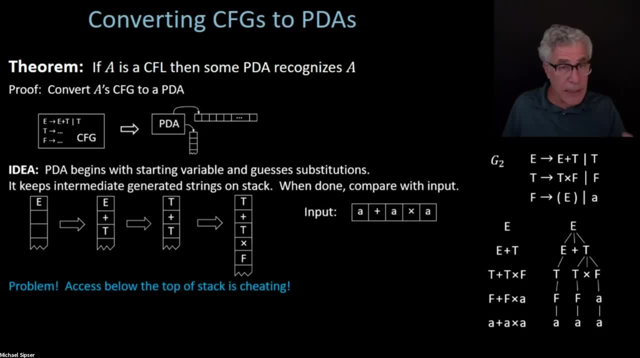 that I described before, without ever needing to dig down into the interior of the stack and doing substitutions there. They're all going to rise up to the top, And we can always do them at the top. So, anyway, I forgot to do that here. 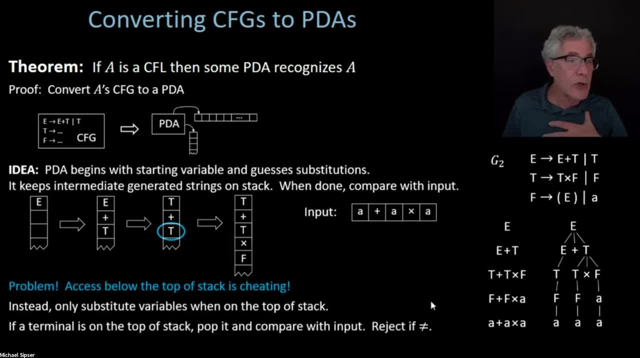 So instead only substitute variables when they're at the top of the stack, Terminals on the top, pop it and compare with the input and reject it if they're not equal. So if you ever have something which is not matching the way it's supposed to, that thread is just going to fail. 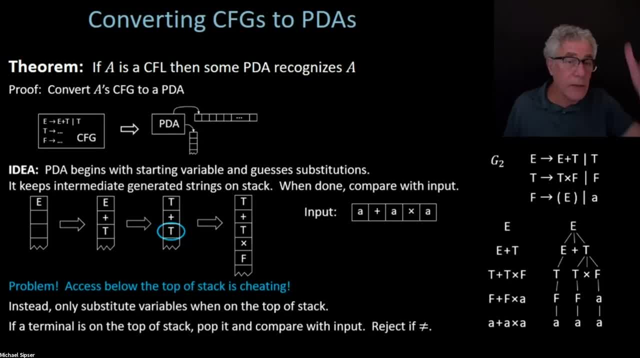 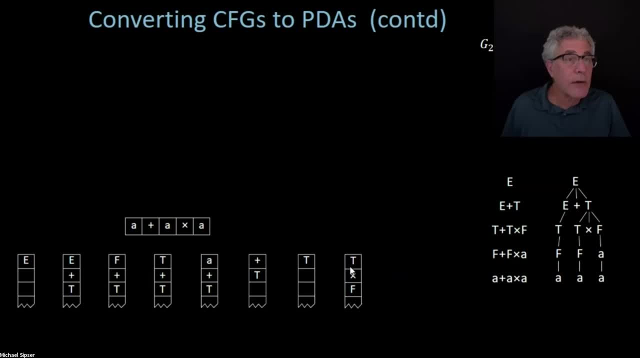 Then there was a bad, non-deterministic choice was made, or maybe the input was not in the language anyway, and there were no good choices. So here, my animation broke here, So let me just put the whole thing up in front of you. 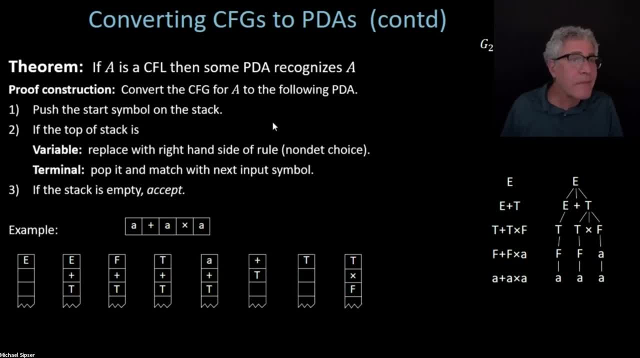 So here is the actual construction: Push the start symbol on the stack. If the top of the stack is a variable, replace it with a corresponding right-hand side, doing a non-deterministic choice among the various possibilities. If it's a terminal, you pop it and match it. 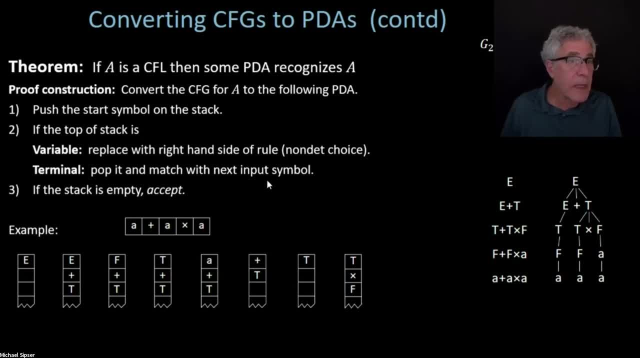 with the next input symbol, And if the stack is empty, you accept. So here is how the stack would actually look for this particular input. It would start off the same, You'd have E and then substitute with E plus T, And then we're going to always do the substitutions. 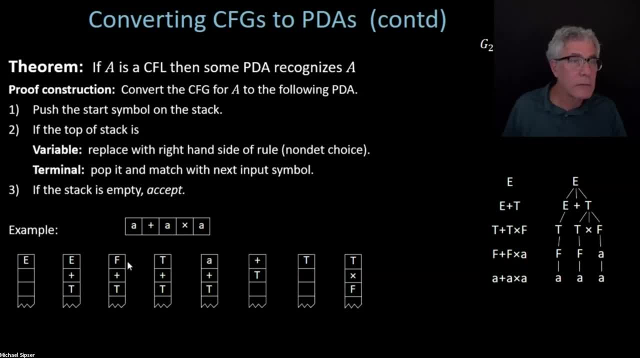 at the top. So E gets substituted by F. Is that right? No, This slide, I messed up, I apologize. So E gets substituted by T, which gets substituted by F. And the point is that when you get to an, A sitting at the top. 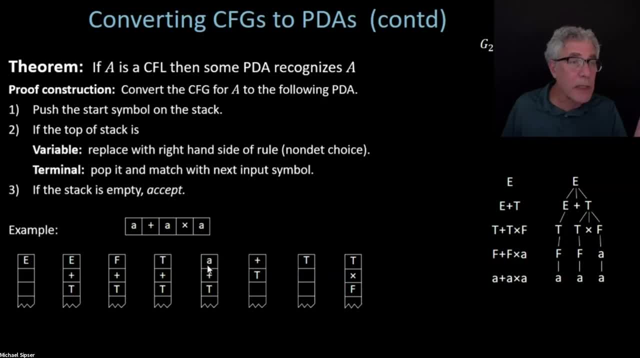 forgive the typos here. now we have a terminal symbol And that's going to get matched off with the next input symbol and get removed, And now we have just the plus and the T left, And then the plus is also a terminal symbol. 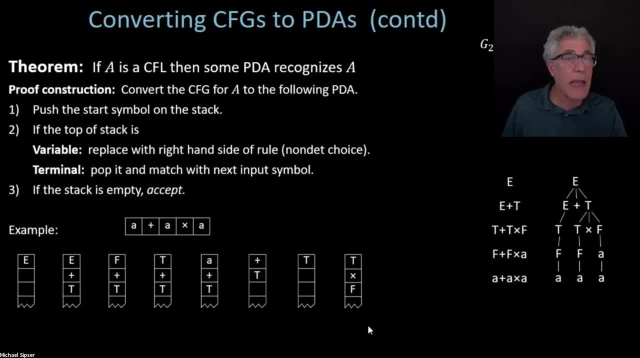 That's going to get matched off with the next thing. We just have a T sitting on the top And now we can do a substitution. OK, so that's how it works. OK, that's all I wanted to say, I think. 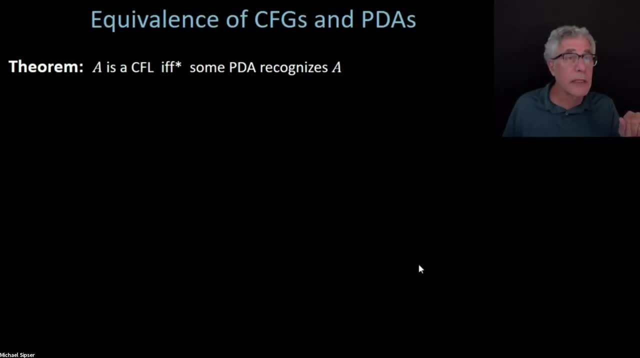 Oh yeah, there's one just remark. So this is not, we're not going to prove this, but I think it's. I do need to say this- that actually you can do the conversion in the other direction too. You can convert a. 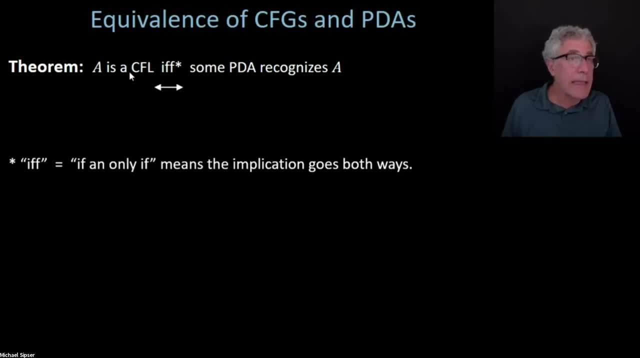 so A is a context-free language if, and only if, some pushdown automaton recognizes A, And if you haven't seen, if and only if. it's an expression I'm going to use again over and over, so you should get used to it. 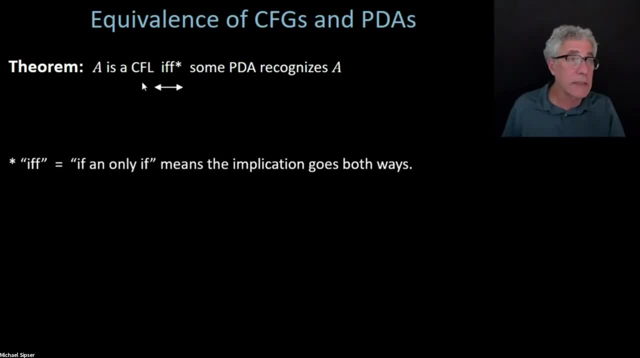 It stands for if and only if, and which just means the implication goes both ways. So A is a context-free language, implies that some pushdown automaton recognizes A and vice versa. So there's really two things you need to prove whenever you have an if and only if. 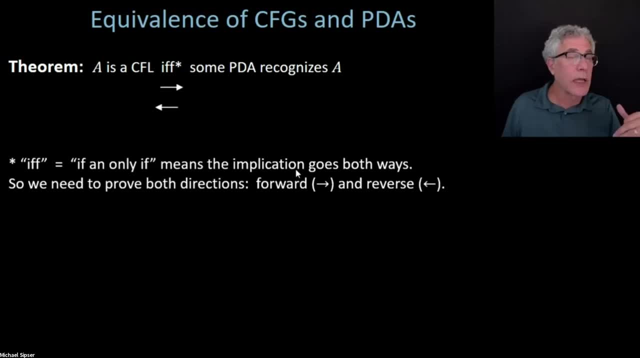 You have to prove both directions. So thinking about that way, splitting them in half. the forward direction we've already proved converting a context-free grammar to a pushdown automaton. the reverse direction we're not going to prove. It's in the book, if you're curious. 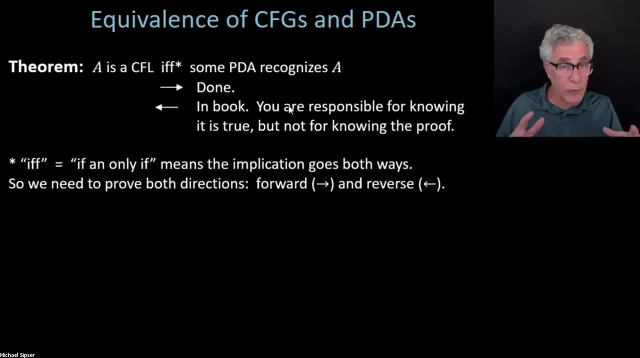 and you are responsible, knowing that the fact is true, but you don't have to know the proof, which is somewhat, a little bit complicated and I think it would take us too long to go through it, so you're not responsible for it. 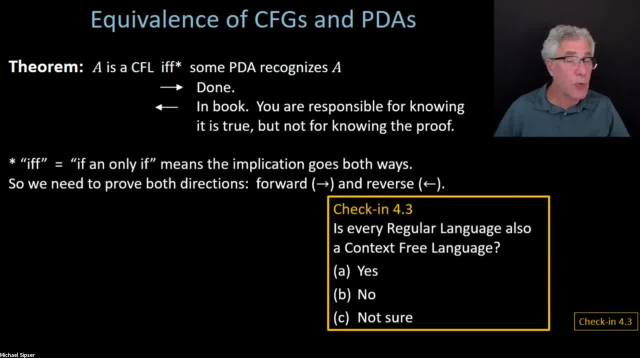 So there's a last check-in here that I have for you, which is just a question which you can answer based on the material that we've presented so far. Is every regular language also a context-free language? Just yes, no, or you're not sure. 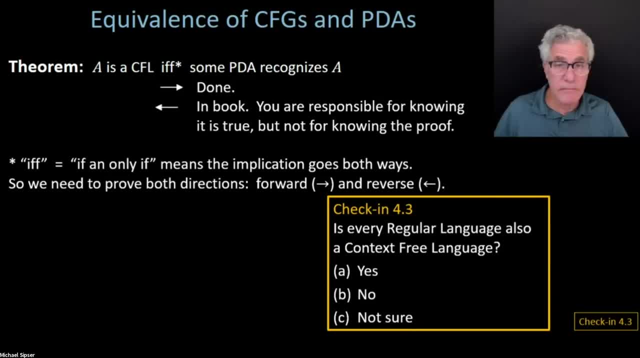 So let me launch that as a poll here. Okay, about to close Ending polling And sharing results. This one, I think you pretty much most of you got. Some of you are not sure. Every language is in fact a context-free language. 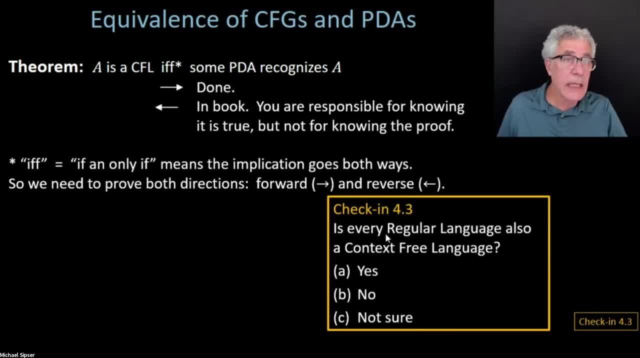 And the way to see that is that every regular language can be done by a DFA or an NFA, as we already showed. And DFA or an NFA is really just a pushdown automaton that never uses its stack, So you can always think of a DFA as a pushdown automaton. 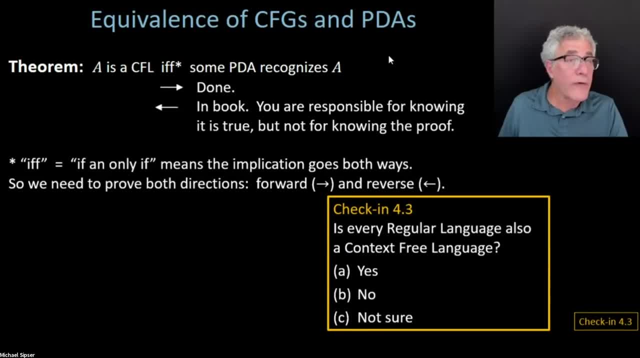 and we already argued that pushdown automata are equivalent to context-free grammars, and so they do the context-free languages. So anything that you can do with a DFA, you can also do with a pushdown automaton, and so is therefore all the regular languages. 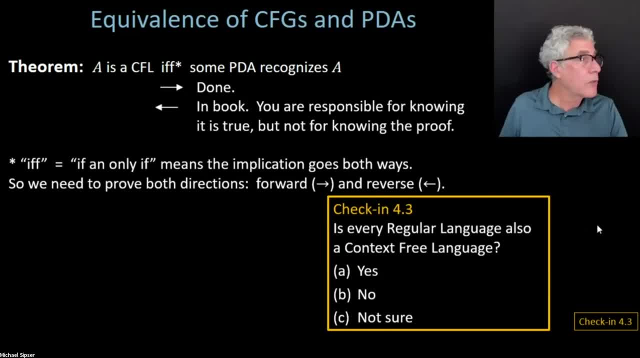 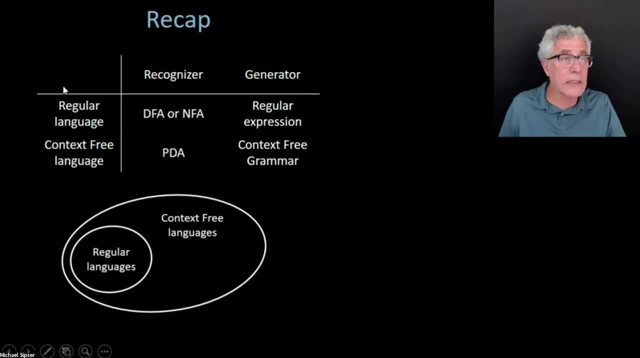 are also context-free languages. Okay, so with that let's just kind of pull things together. A little quick recap of what we've been doing so far in the class. We have the regular languages and the context-free languages. We had the two forms of sort of getting at them. 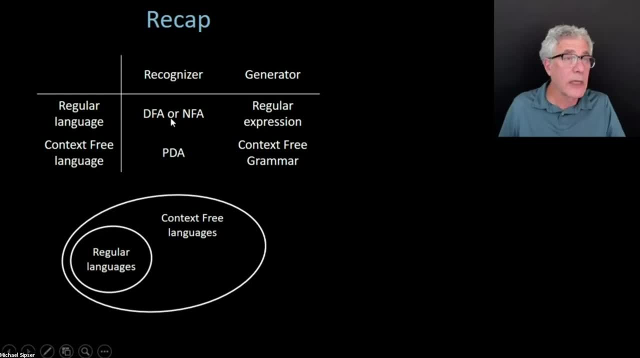 the recognizer form, which is like the automata-based perspective, like either a DFA or an NFA in the case of the regular languages, the pushdown automaton for the context-free languages and for the generators, we had the regular expression for the regular languages. 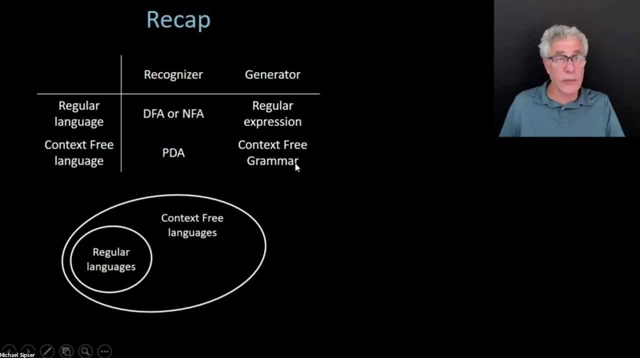 and the context-free grammars for the context-free languages. Okay, And, as we just pointed out in our last check-in, the regular languages form a subset, and in fact a proper subset, of the context-free languages, as shown in this Venn diagram. 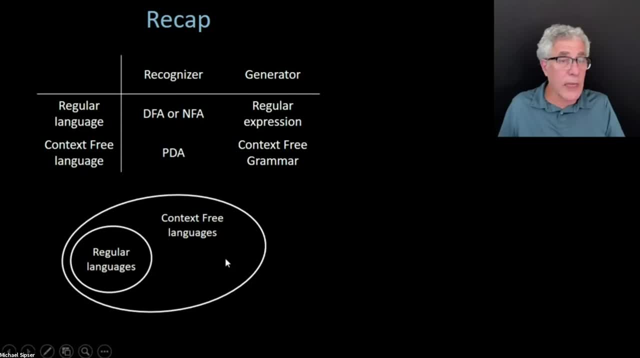 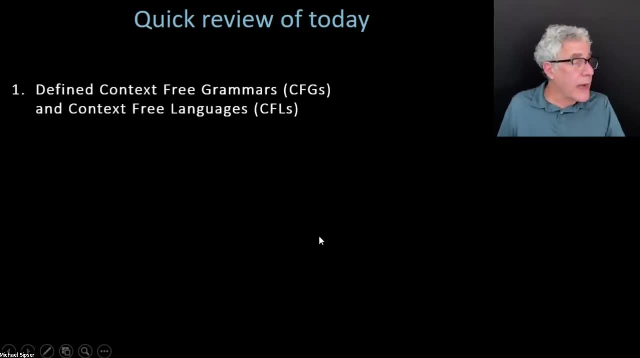 because we have already exhibited languages that are context-free but not regular. All right, So quick review: We've defined the context-free grammars and their associated languages, the context-free languages. We defined pushdown automata and we showed how to convert context-free grammars. 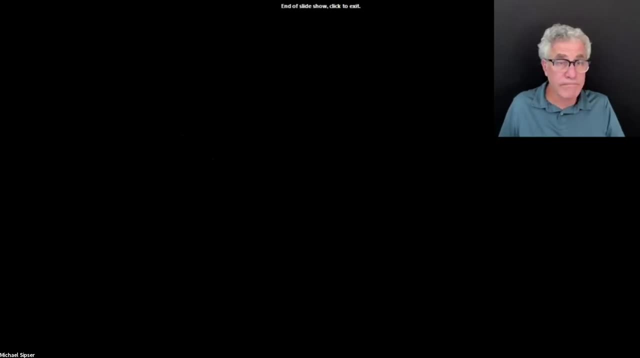 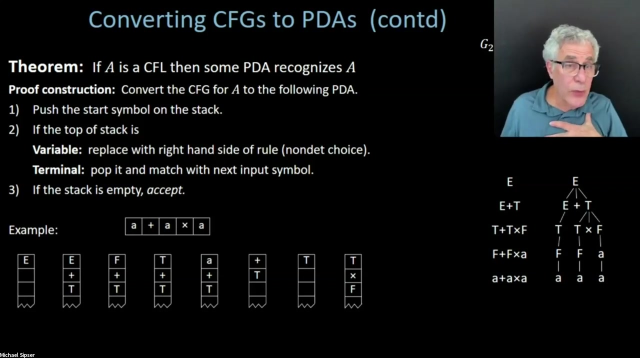 to pushdown automata, And that's all I have for you today. Okay, here's a question I'll answer to everybody. Why do we restrict ourselves to a stack? Why don't we use random access memory? We will use random access memory. 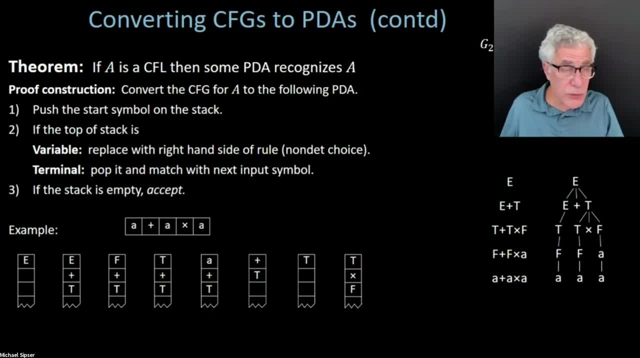 for the next model called the Turing machine, and we're going to introduce that, I think, next lecture. So that's going to be the model that we're going to stick with throughout the term. But we have not. we will kind of use introducing weaker models. 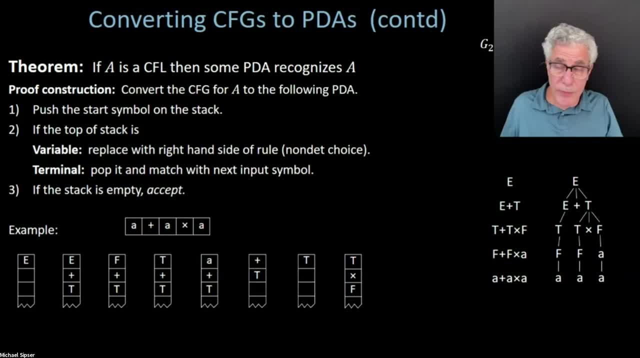 as a kind of a prelude to the more general purpose computational model, really to get ourselves warmed up, and also because for the weaker models, you can fully analyze them in a way that you cannot for Turing machines. We'll be able to, as you will see. 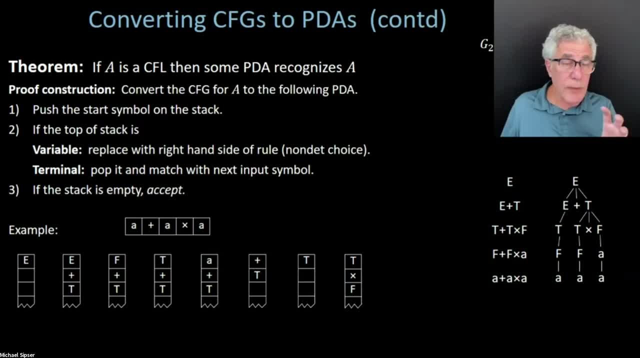 you can determine properties of languages for the weaker models that you cannot for the more general models, And so I think that's helpful to have that perspective that for some cases you can get a full analysis and some other cases you cannot. But anyway, 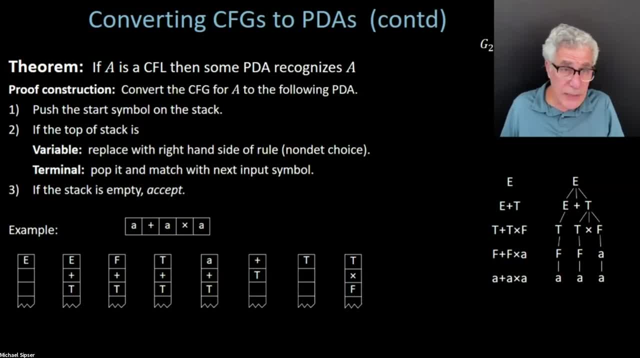 that's the reason why we restrict it to the stack, besides the fact that these models have applications that I think are worth people seeing. Why- yeah, some reason- we chose a stack. Well, why did we choose a stack and not some other data structure?